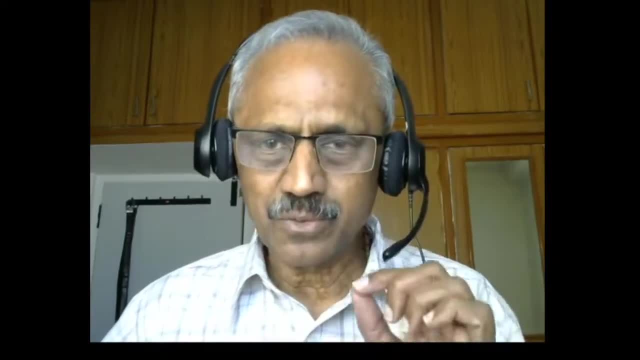 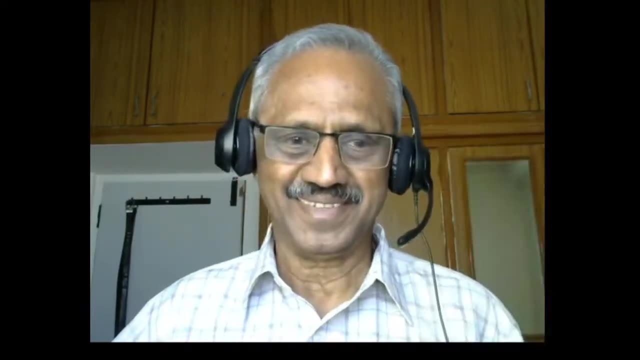 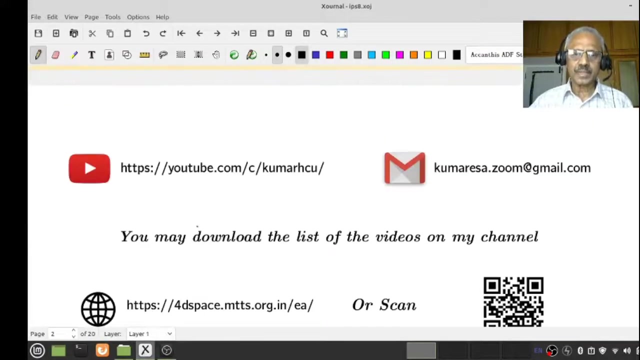 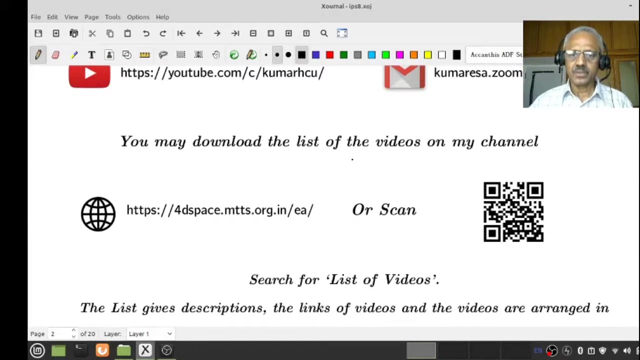 This is the trick. I hope you all enjoy it and you really find it's very, very easy, just because geometry is clear in our mind. Let's get started. This is my channel. this is the email ID. you can download the list of videos from here or you can scan this. 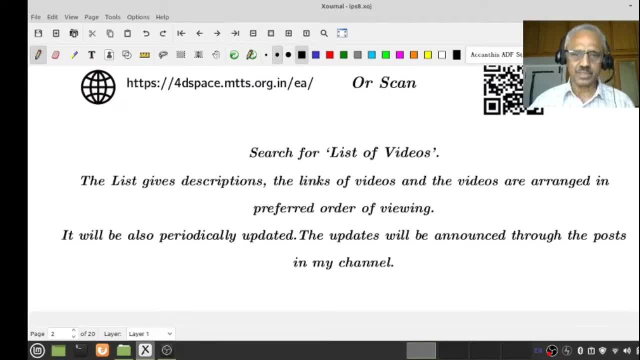 What is the advantage of having the list of videos? It gives you description, it gives you URL, it also gives references and also, for example, inner product spaces. this is the eighth lecture. all of them will be ordered in the fashion so that you know where to start. 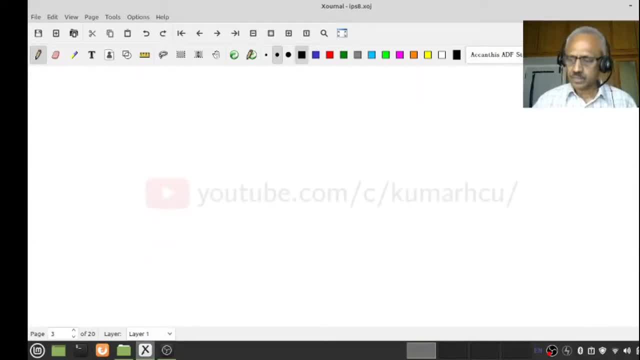 Okay, that's the advantage. Okay, let us quickly start. Let's start the problem. so let V be an inner product space, possibly over R or Rc. okay, it does not matter where we are. okay, you will see that. okay, it's a complex conjugate. okay, the other variable, second variable, etc. will not appear. everything is easy. 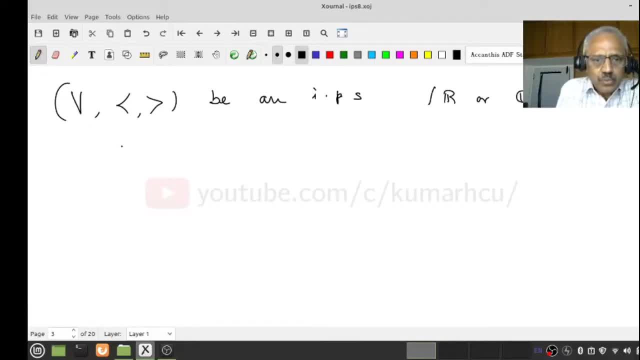 So what are the things I want you to remember? Suppose V- okay- is a vector, V is a vector, non-zero vector and X is any vector in this- okay. I will always draw a picture like this: this is my X and this may be my- oh, sorry, this is my V, this is my V, this may be my X and I want to automatically project it on this. 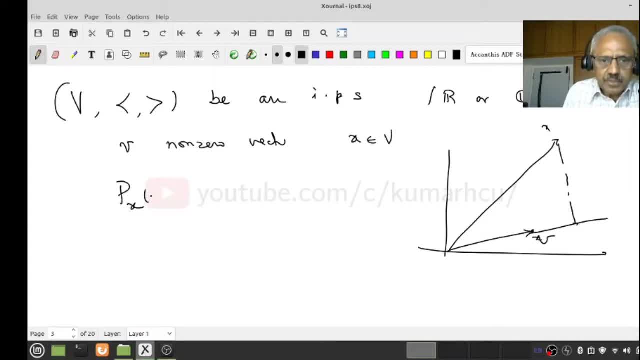 Okay, so orthogonal projection. we denote by PX of V. what is this beta position? let us recall: this is V minus you project this. okay, the orthogonal projection is X inner product, V by norm, V squared into V. okay, just ignore all these things. these are orthogonal projection. okay, this is this vector. 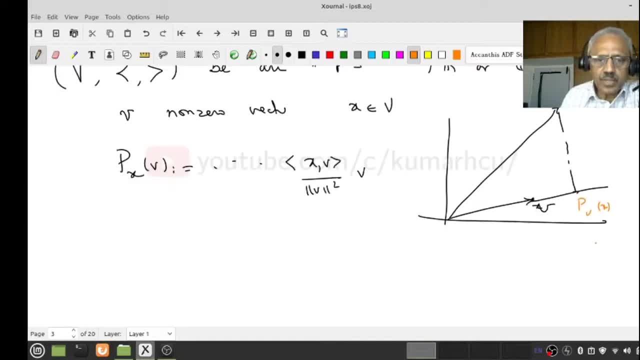 P, V of X. right, what do we have learned? So this is the first definition. recall this. and second thing you should recall is this: X minus PX of V, okay, this inner product with V is zero, that is, X minus PX of V is perpendicular to V. that is this object. 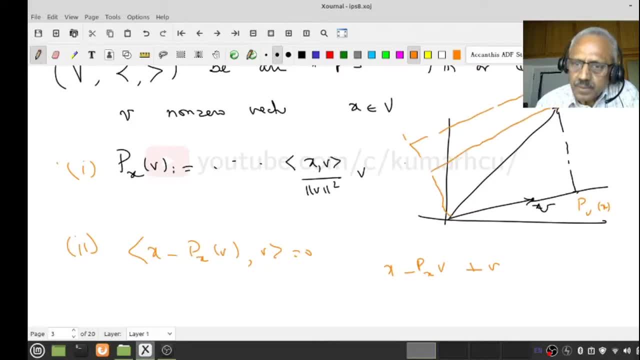 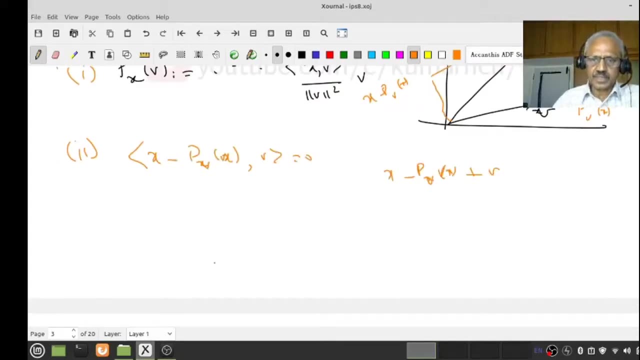 Sorry, this is not a good thing. this may be my X minus PV of X. again, I am writing wrongly PV of X. orthogonal projection. okay, remove the orthogonal projection right. these are the only two facts I will need. 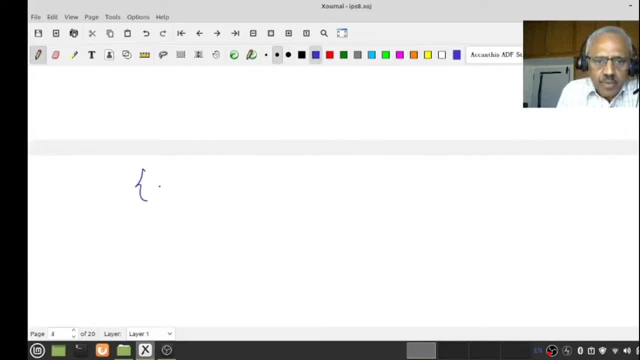 Now let us assume V1, so let us assume our this space dimension is N. okay, let V1 to V2.. V1, be a basis, V. what do you want to construct? idea is to construct an O, N that is orthonormal basis. let me see whether I have switched on the recording there. it is on, okay, and also I am sharing, right, yeah, basis. what does it mean? that is, I want to construct a basis. 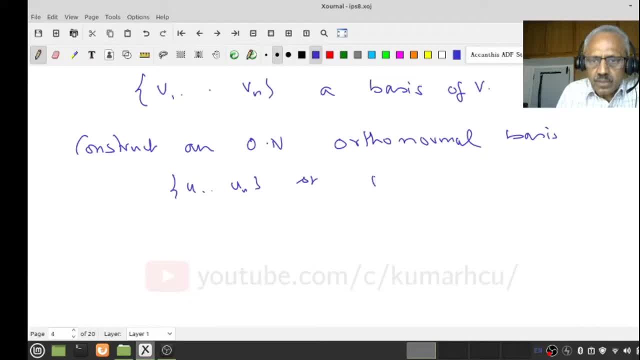 this is U1 to Un, so that norm of Ui, Uj is 1 for all j and inner product of Uj with Uk is zero for j, not equal to k. If you know the Kronecker delta, then Uj- Uk inner product must be delta jk. this is called Kronecker delta. 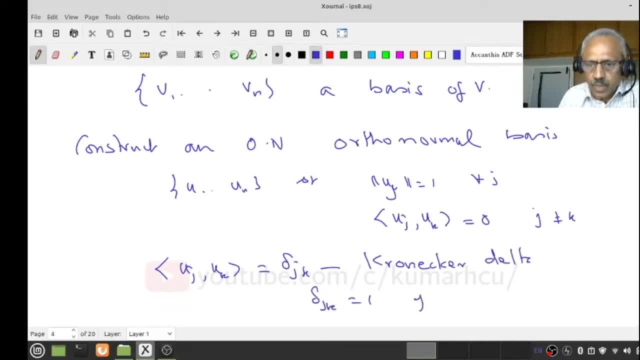 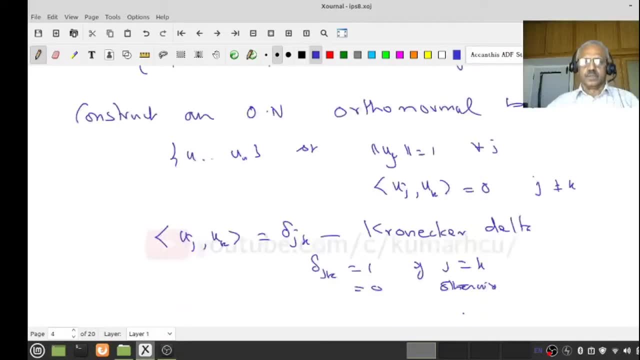 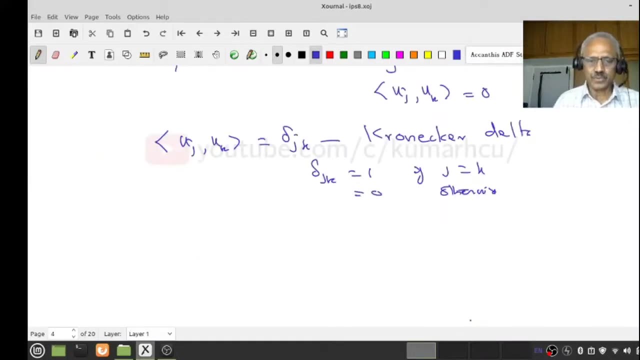 That means delta jk equal to 1.. j is k and equal to zero, otherwise, Okay this because you should learn some jargon also on the way. right, okay, right, okay, now you want to do that. 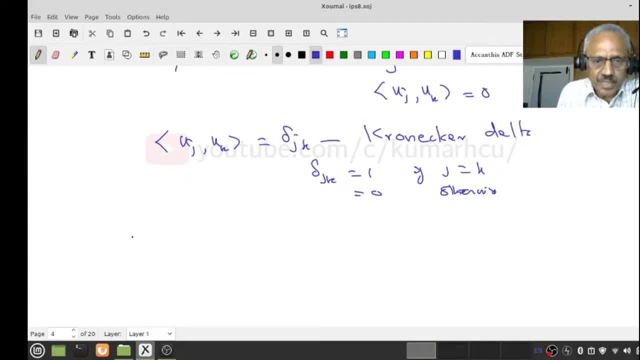 So the first thing let us set up to make my life easy. when I want to project some vector x and b- okay- onto vj component, okay. So instead of pvj of x, I will write as pj of x, right, so that I do not write pj of x. and what is pj of x? this is x, inner product, vj, vj and norm- vj, vj. 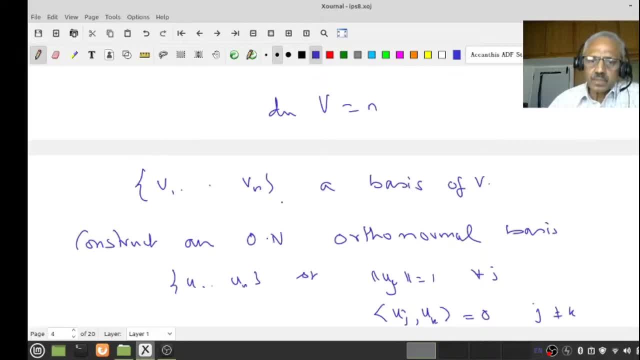 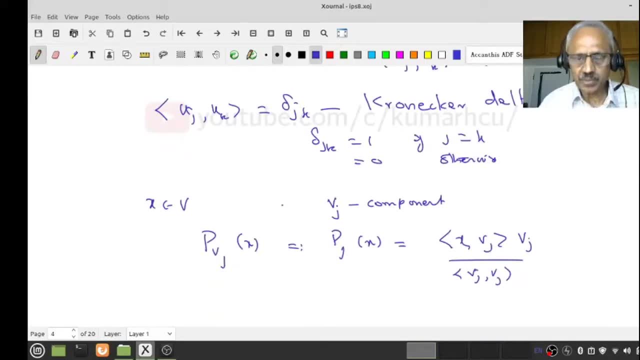 Now notice that vj's are all elements of a basis. therefore, none of the vj will be zero. therefore, I can write it in the denominator inner product, vj, vj, because it will not be zero. Okay, right, so how do we do that? 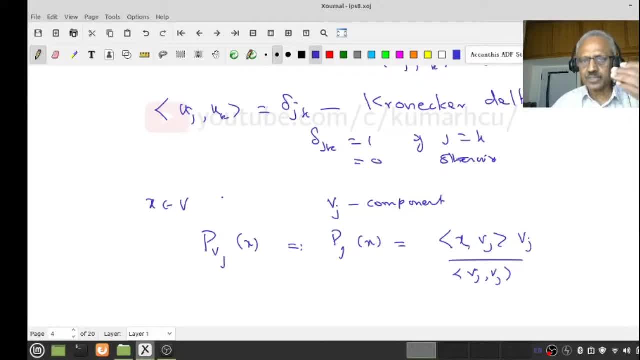 Let us say: go through, see again. so far I have not used whether it is inner product over r or c. you will see that I am just using inner product symbol only, right, okay, now let us go to the next one. okay. 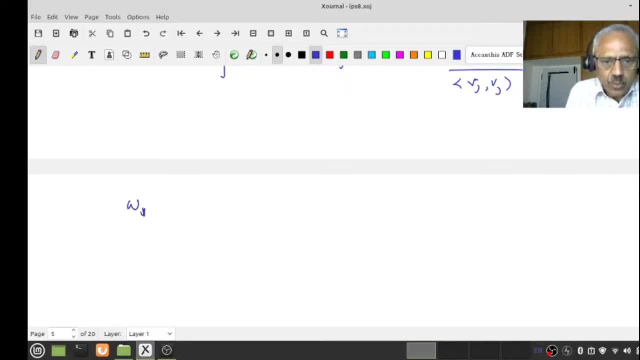 So what we do? so I will take wj, w1 equal to v1, so I do not change it. no change at all. okay, now I want to do w2, now recall how do you do that? so let me just write this as v1. 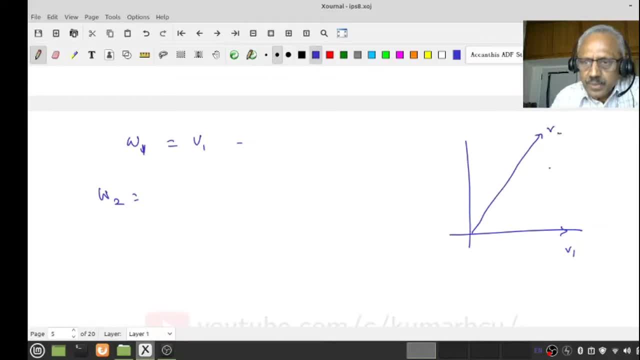 And this is my v2, then what do I do? I want w2, that should be orthogonal to w1,, that is, it should be orthogonal to v1, and do you know how to construct it? yes, you know how to construct it. how do you construct? from w2, you take away p1 of w2, right, just in case you had forgotten, this is w2 minus w2, v1 by v1. 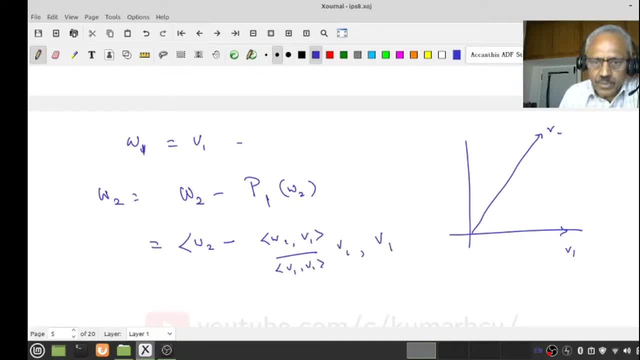 Then v1, v1, and this inner product v1,. okay, w2- inner product v1 will be this, and this will be w2- v1 minus w2, v1, v1, v1, v1, v1,. therefore, it is w2- v1,, is that okay? therefore, it is 0.. 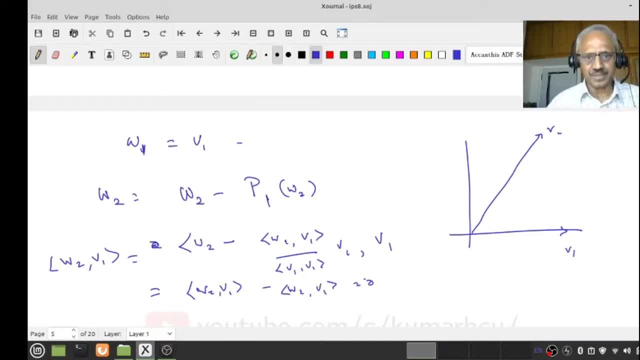 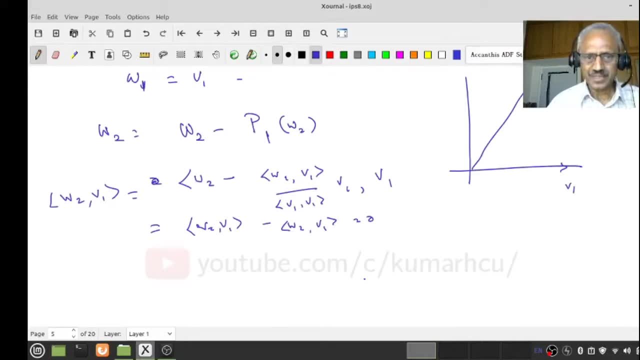 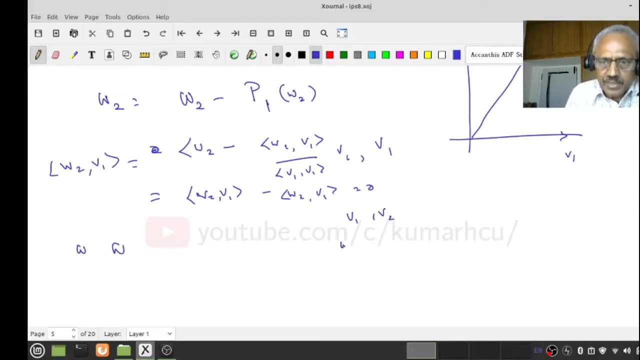 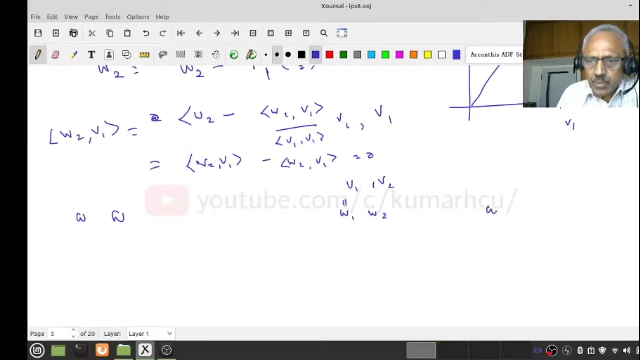 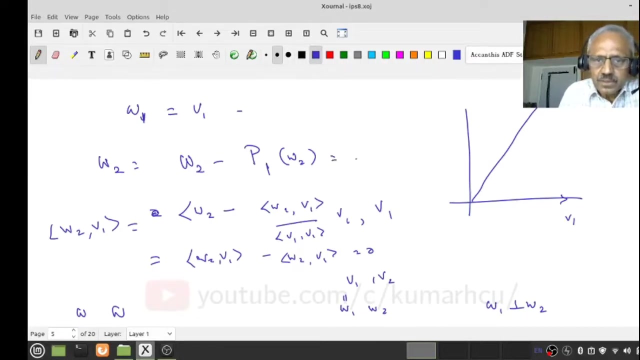 So did I use its real inner product or complex inner product? nothing, because this we have checked for any inner product. okay, be it real or complex, is that clear? so I got a w2.. Okay now, what do I have from v1, v2,? I got a w1, w2, what is w1,? is this? what is w2, as defined right, and what do I know? I know w1 and w2 are orthogonal to each other. okay now can w2 be 0, suppose w2 is 0, go back to the definition. what does it mean? this is this: is w2, my sum. scalar times. 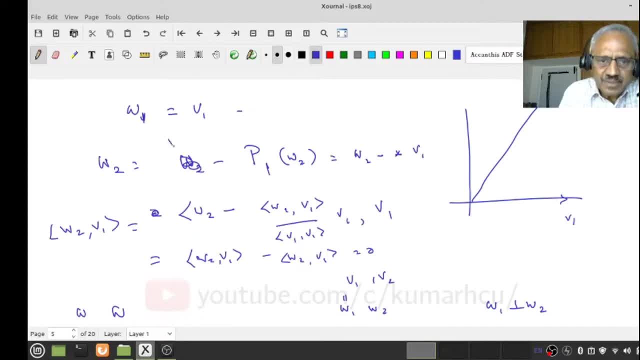 v1, oh sorry, again v2, here I wrote correctly v2, v2, v2, w2 is v2 minus p1 of v2,. I am sorry for the goofing again. let us quickly look at that. what is my w2, w2 is v2, p1 of v2, that is. 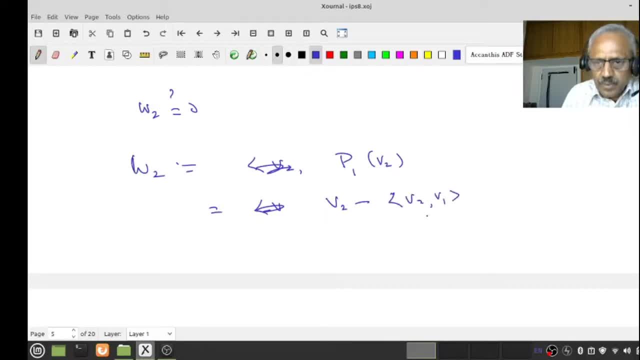 v2 minus v2, v1 by v1, v1, v1,. okay, and what did we check? w2 and w1 is 0, that is same as saying w2, v1 is 0, okay, just just now we checked it. okay, right now. now can w2 be 0, if w2 is 0, do that? what do what do you get? you see, this is 0, right-hand side is 0, that means v2 is a linear. 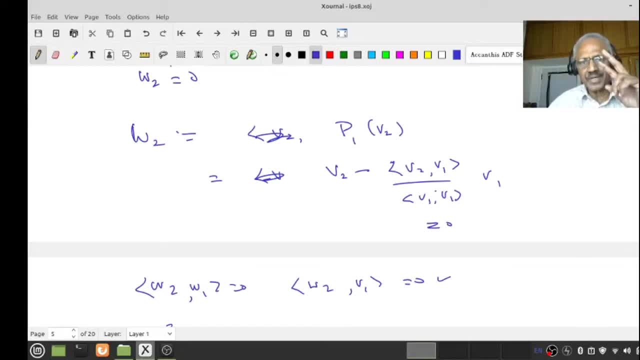 is a scalar, is a scalar multiple of v1, that means v1 and v2 are linearly dependent. but where do v1 and v2 come from? they come from a basis. therefore, it cannot happen, do you understand? therefore, this cannot happen. therefore, w2 is not 0,. right now, let us look at next one. now, let now see notice that w2 belong to the span, the linear span, of v1 and v2,. 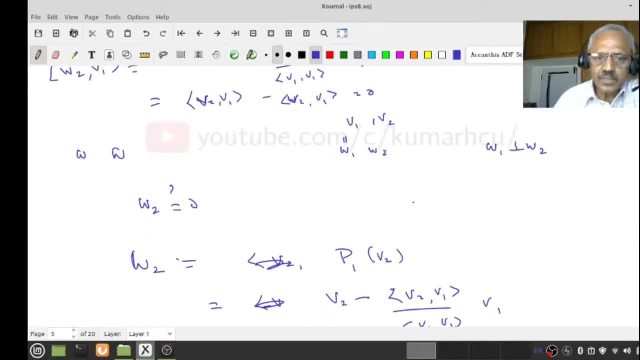 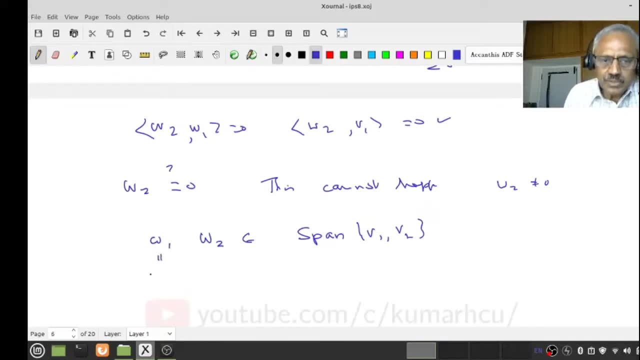 yeah, because look at that, what is w2, v2 minus scalar multiple of v1, right? and w1 is also there, because w1 is nothing other than v1, you understand? therefore, what do I conclude? span of v1, v2, and span of w1, w2,. okay, so this contains this, because w1, w2 belong to this. 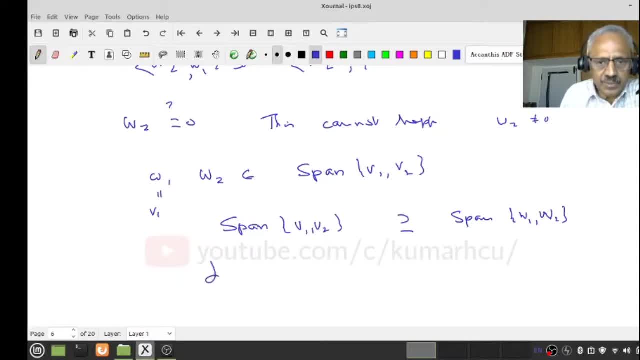 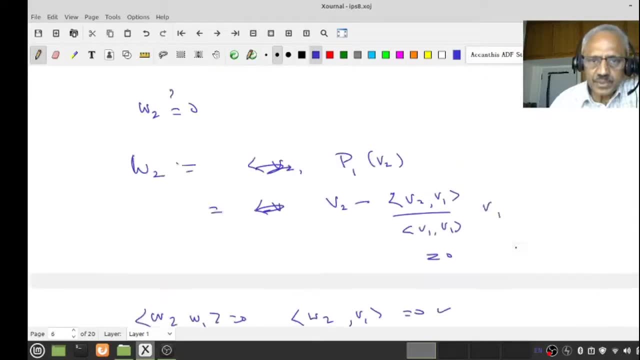 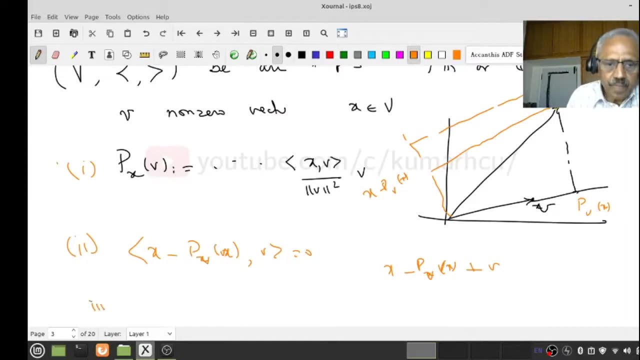 is that clear? now? what is the dimension here? dimension is 2,. right, and remember the third fact I needed. I should have said that I forgot. yeah, third fact here is: if w1 to wr non-zero vectors, vectors are that. 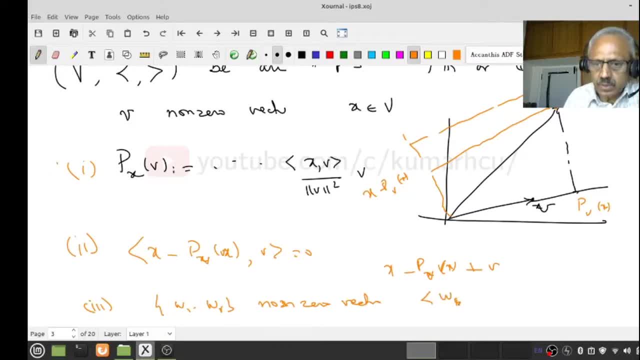 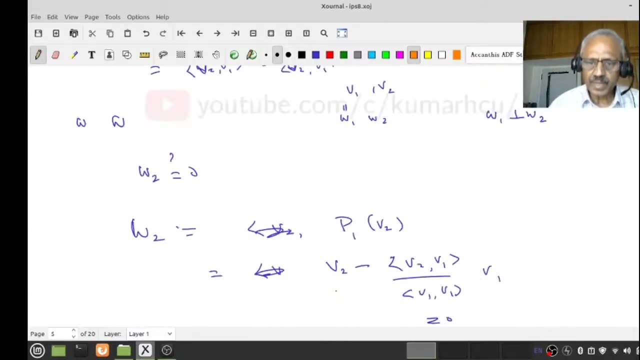 w, wi. wj is delta ij, then this is a linearly independent. this we saw in the last lecture, right? okay, therefore, let us come back. so what do I think I have concluded, so this dimension is also 2,. 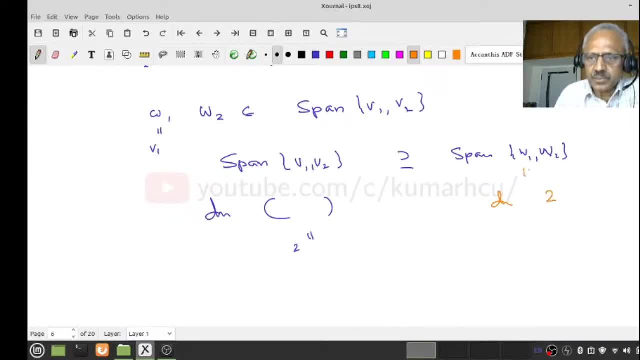 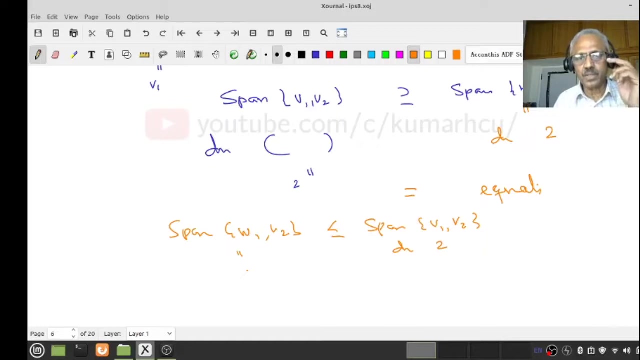 what are you following? dimension of this fellow is also 2, and that is a subspace of this space which is of dimension 2, therefore equality holds. you understand that that is span of w1, w2 is a vector subspace of v1, v2, since this is linearly independent, this dimension is 2, and since w1, w2 are non-zero and orthogonal to each other- we have already seen any orthogonal set consisting of non-zero vectors is linearly independent. therefore, this dimension is also 2, therefore we have these two are equal. 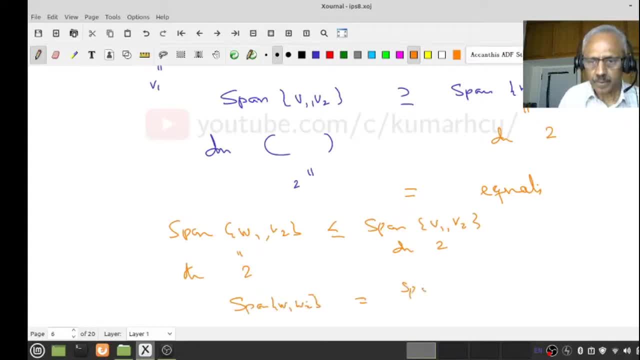 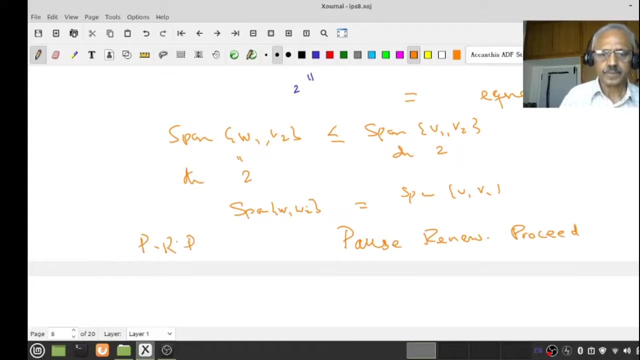 okay, pause, review, proceed. so now, how do I define w3,? remember, w3 must be perpendicular to w1, and w3 must be perpendicular to w2, now how do you think I will get it? I should get it from v3,. 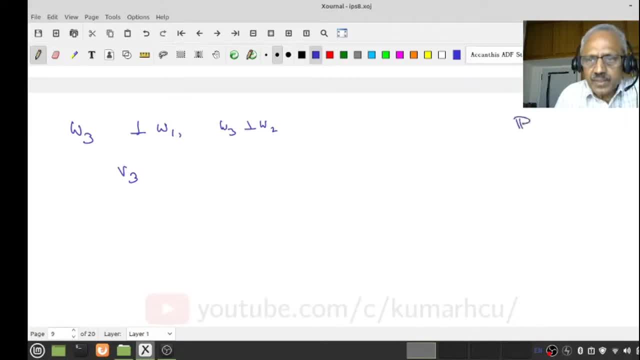 how will I get it from v3, remember, in r3 with the dot product? okay, if I have abc, okay, so call this as vector x, then x dot e1 will give me a and x dot e2 will give me b. 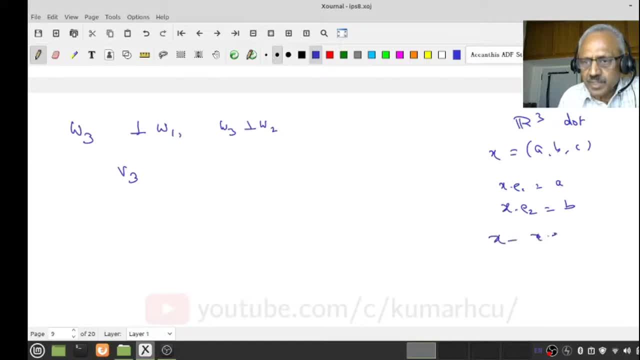 therefore, if I throw away from the vector x x dot e1, e1, plus- sorry- minus x dot e2, e2, what i will get will be 0, 0 b, which will be perpendicular to e1 as well as perpendicular to e2. 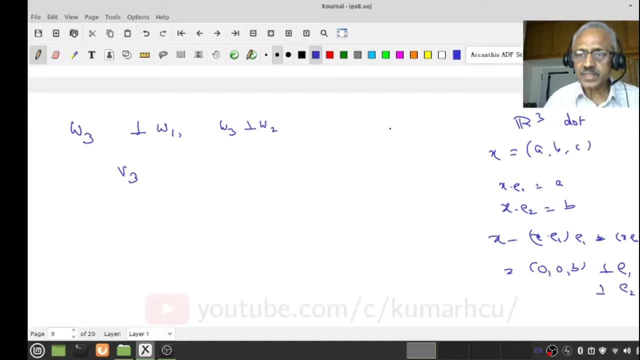 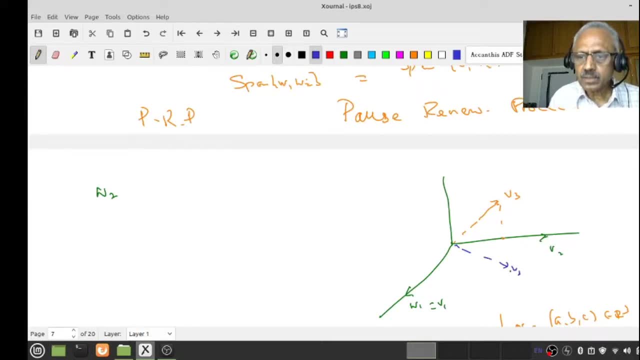 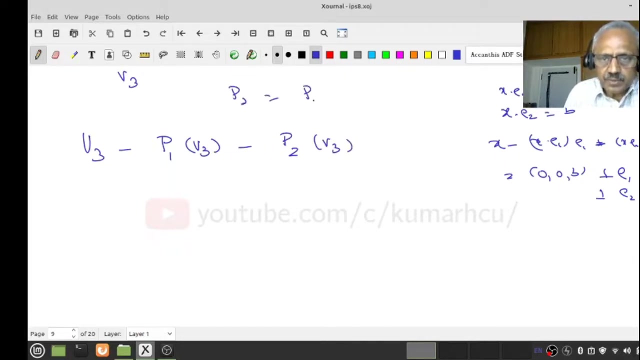 right, so the same thing. so what? as i said in the picture earlier, okay, i am taking w v3 projecting onto the w, w2 and w1 component. okay, therefore, from v3, what do i do? i start with p1 of v3, right, minus p2 of v3, where p2 is the projection with respect to w2, not with respect to v2. 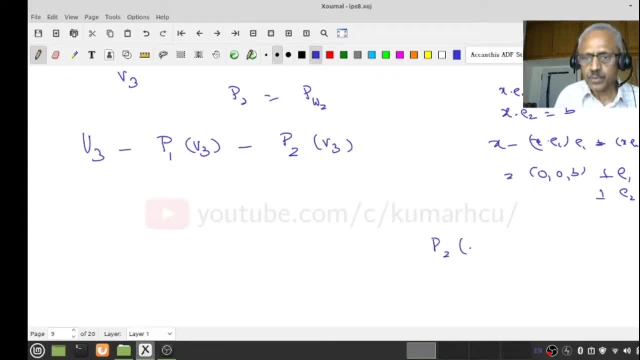 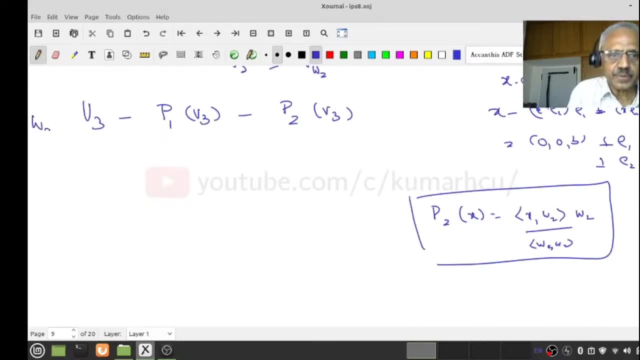 you understand that. what is the projection of p1, of v3, p2, of X? this is X, w2 and w2 by w2- w2. you understand that? okay, now this is my w3. so again, to think geometrically, from v3, I am taking over the w1 component. I am. 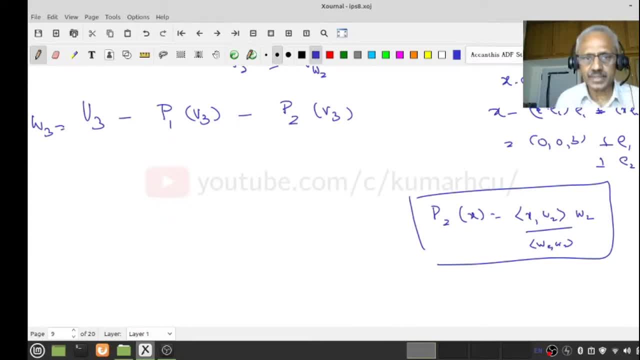 also taking the w2 component, not v1 v2 component. okay, then I, what I get should be perpendicular to as W 1 as well as w2. right, that's it. notice that this is something some scalar multiple of w1. this is some scalar multiple of w2. are 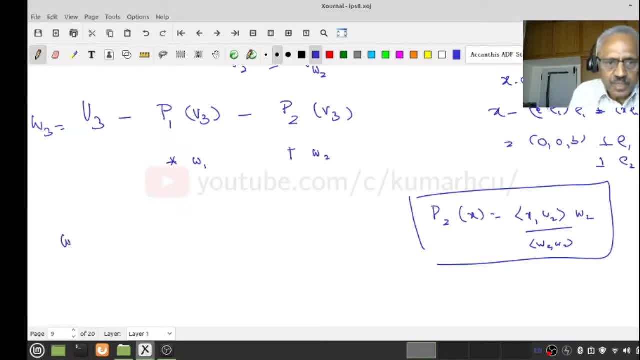 you following, because that's a crucial thing I want to do. therefore, w3- inner product, w1- what is it? some scalar mut? okay, right, this is I want to say: this is 0. therefore it is v3. what do I have? I have w1 minus p1. what is p1? that I know? that is nothing. 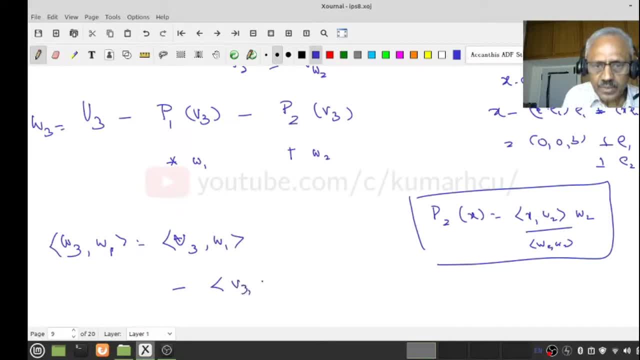 other than v3, w1 by w 1, w1, w1. okay, and inner product of you next will be v3 w w2 minus w 2, w 2, w 2, inner product w 1, because I am talking starting with w 3. 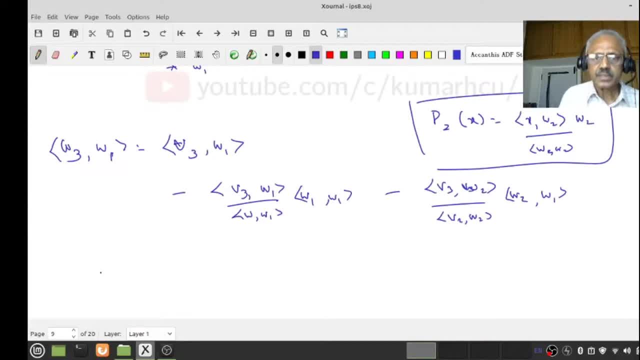 you understand. now let us look at this right. this one get cancers. therefore, I have W 3, V 3 minus W 1. okay, they add up to 0 and this fellow, W 1 and W 2, are orthogonal to each other. therefore, this fellow is 0. 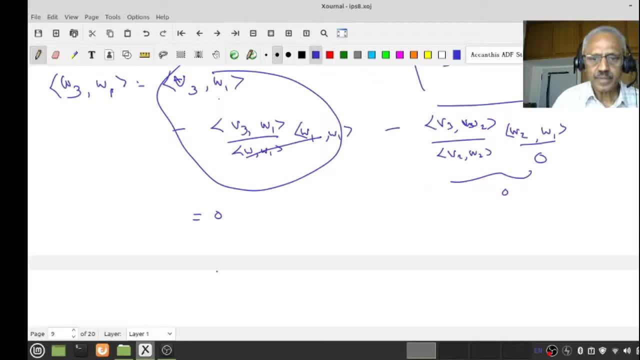 therefore, this term is also 0. therefore, I have proved this right. similar way. similarly, if I take a 2, I will put a 2 here, 2, 2 and I will have a 2 right. therefore, this will be 0. are you following W 3 minus W 2? sorry, inner. 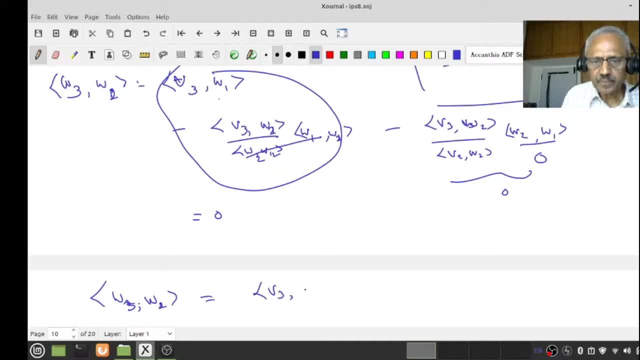 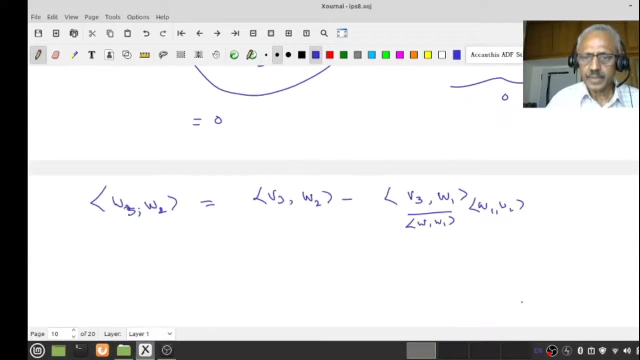 product W 2 will be V 3 W 2 minus V 3 W 1 by W 1 W 1 W 1 W 2 right minus V 3 W 2 minus W 1 W 2 right minus V 3 W 1 by W 1 W 2 right minus V 3 W 1 by W 1 W 2. 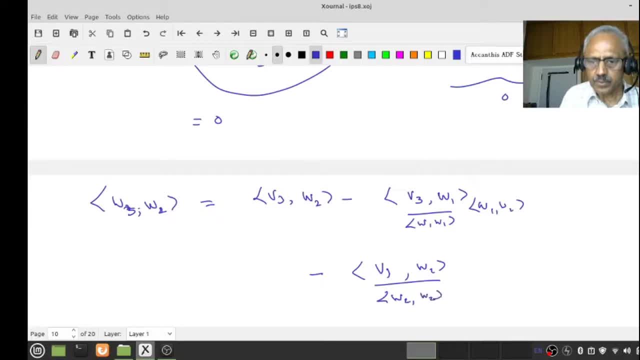 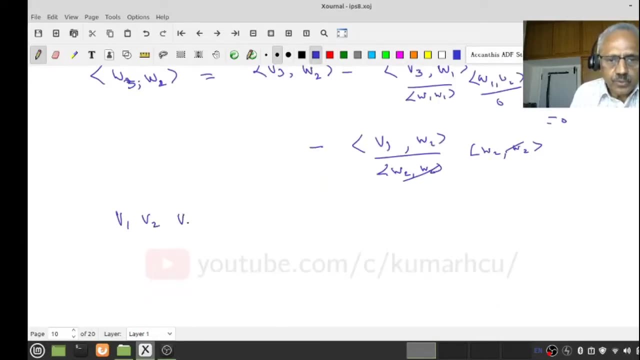 W 2 by W 2, W 2. inner product: W 2, W 2. you follow that and this is 0 and this cancels, so I get this equal to 0. are you following so what I have shown? so, from V 1, V 2, V 3: okay, I have constructed W 1, W 2, W 3. okay, this is orthogonal, okay, set. 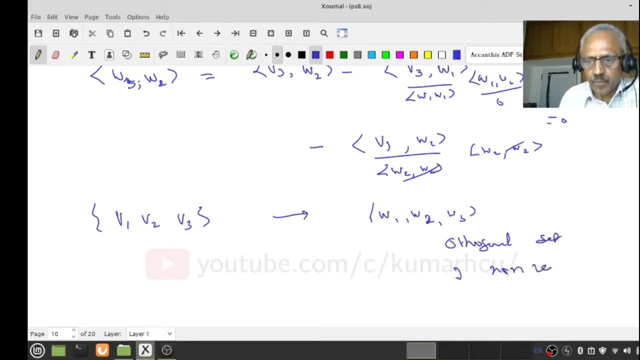 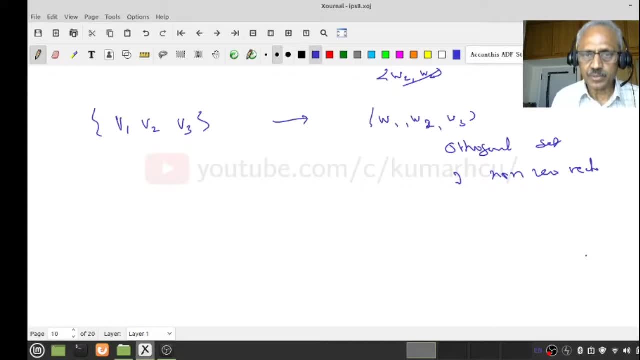 of nonzero vectors, because we already saw: W 1, W 2, W 3 are nonzero and they are mutually perpendicular. they are not earth or normal. I am not playing, they are not more. do you understand that? they are just simply orthogonal to each other, right? therefore this set is linearly independent, right? so, like last time, 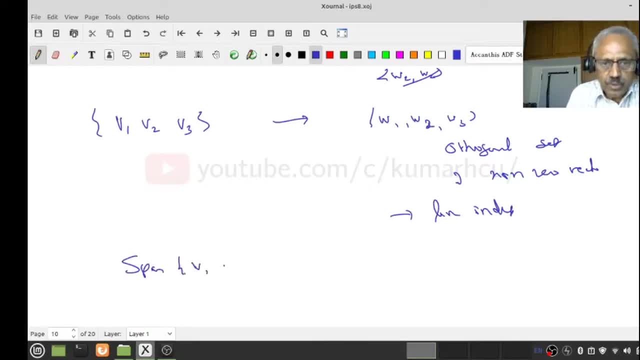 therefore, span of W 1, W 2, W 3, remember, W 1, W 2, W 3 are not orthogonal to each other, right? so, like last time, therefore, span of W 1, W 2, W 3, remember okay, if I have W 1, okay, then that belongs to span of V 1, V 2, V 3, because I 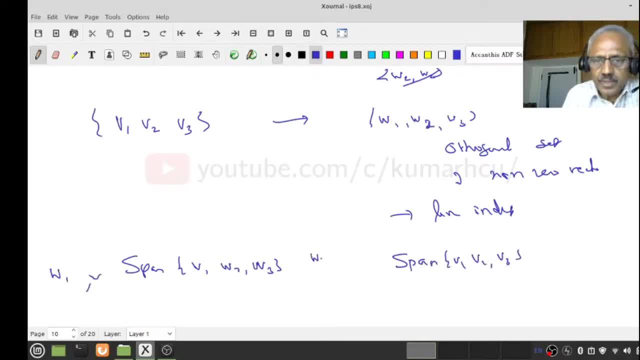 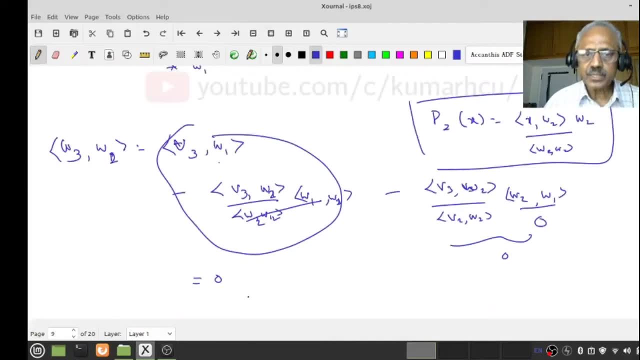 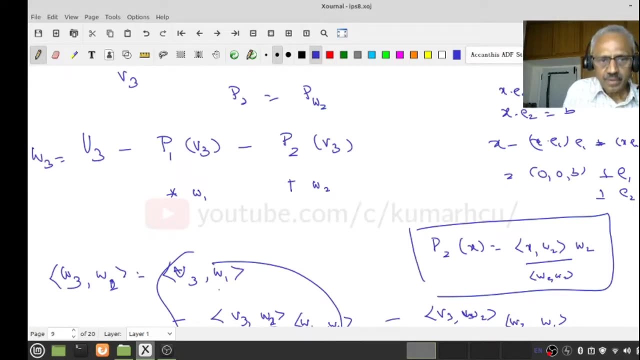 already know, W 1 and W 2 are here. all right, it is in the span of V 1, V 2. now let's look at W 3. now, what is W 3? W 3, as we saw, is a linear combination of V 3, W 1 and W 2. 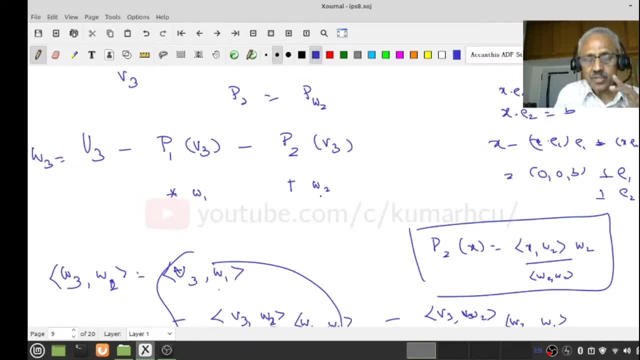 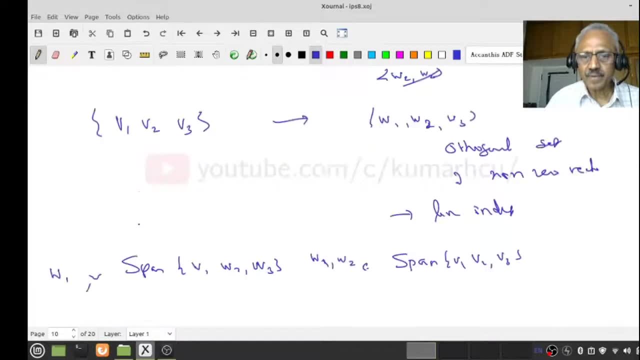 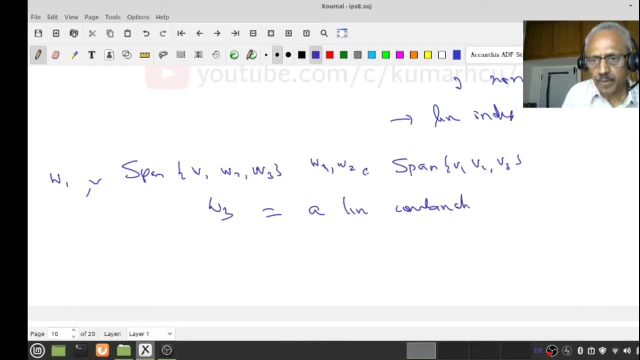 but W 1 is nothing other than V 1, but W 3 is a linear combination of V 1 and V 2. you understand that, therefore, this W 3 is a linear combination of V 1, V 2, V 3. right, and we know W 1, W 2 already belong to span of V 1, V 2 and hence in the span of 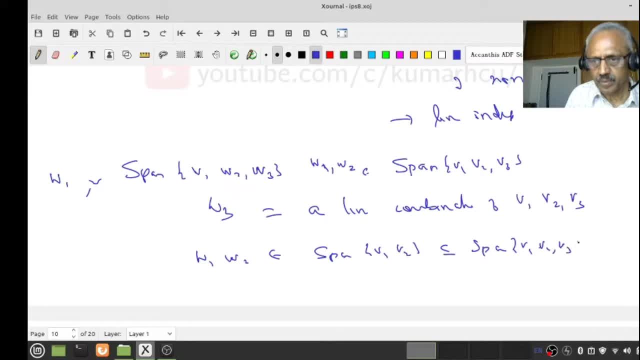 V 1, V 2, V 3. therefore, what is the conclusion? therefore, span of W 1, W 3 is span of V 1, V 2, Z, v3. so understand this. if i understood this much, the rest is very trivial induction. we will do that. 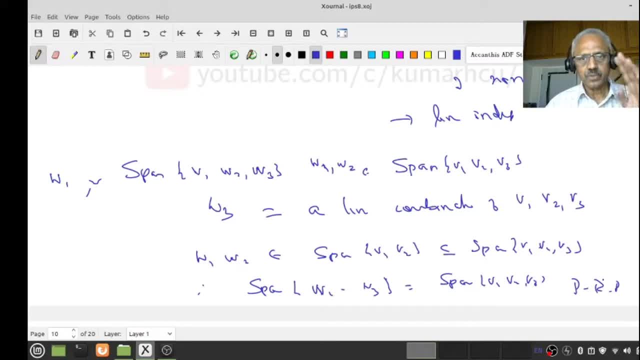 okay, please stop. go through how we constructed w2, how we consider w3. important thing is w3. okay, because when i consider w2, i simply have to project onto the w1, which is nothing other than b1, but when i wanted to consider w3, i have to project v3 onto w1 and w2. that is, i have to. 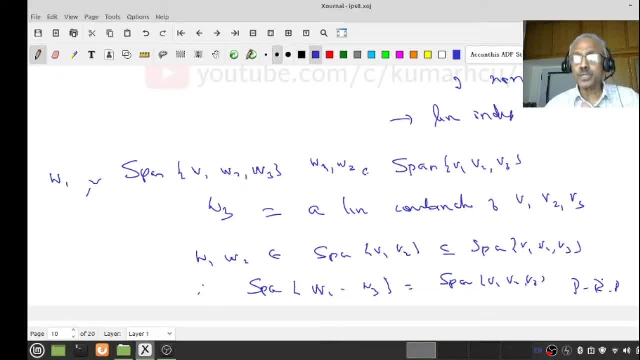 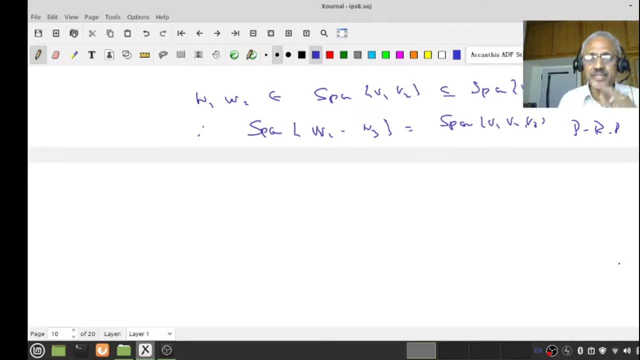 subtract from b3- w1 component and w2 component, not b1- v2 component. keep that in mind, because w1- w2 are already orthogonal. that is why i can construct whatever i get, as w3 is orthogonal to w1 as well as w2. okay, this is the beautiful geometry. understand that? 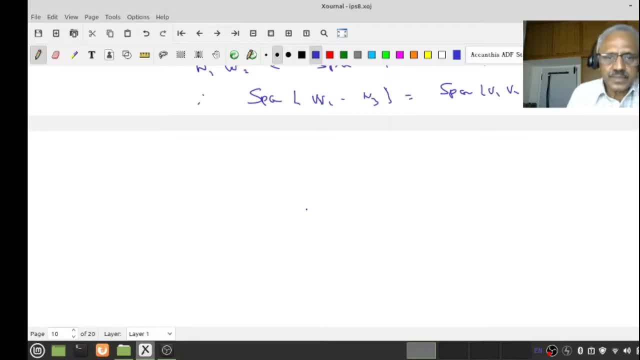 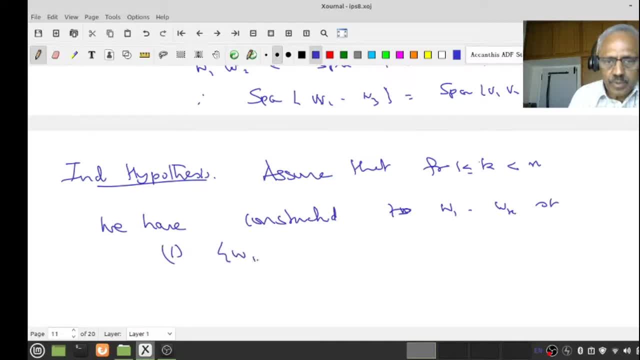 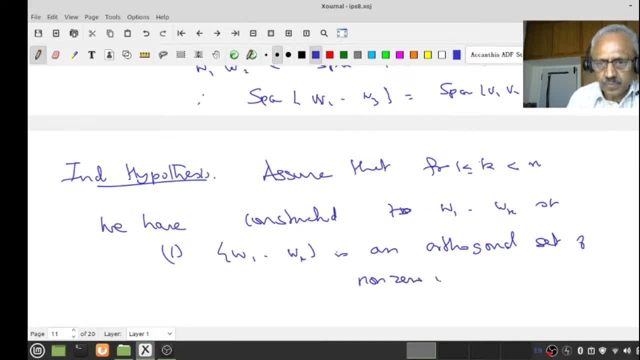 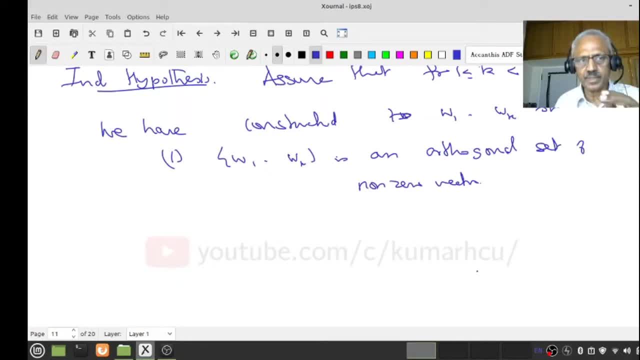 later also orthogonal. what does it mean for i not equal to j or for i and j wi, for i not equal to j or for i and j wi, for i not equal to j or for i and j wi? inner product wj will be delta i- j. 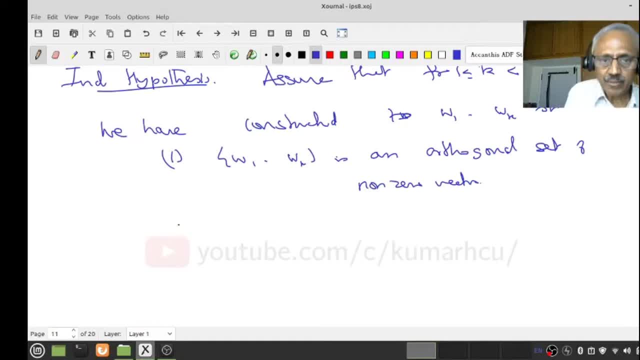 inner product wj will be delta i j. inner product wj will be delta i- j, where i and j run from 1 to k, where i and j run from 1 to k, where i and j run from 1 to k. and what is the second one? the second one. 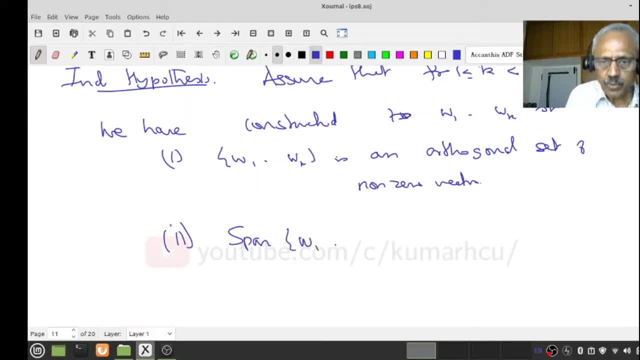 and what is the second one? the second one and what is the second one? the second one is the span of. is the span of? is the span of w1 to wk is same as the span of w1 to wk? is same as the span of w1 to wk is same as the span of v1 to vk. 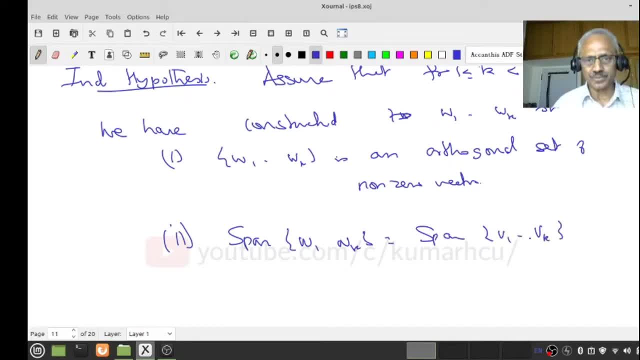 v1 to vk. v1 to vk. we are done it for we are done it for. we are done it for one, two, three up to three words: one but one, two, three up to three words: one but one. two. three up to three words: one, but for induction it's enough if i was done. 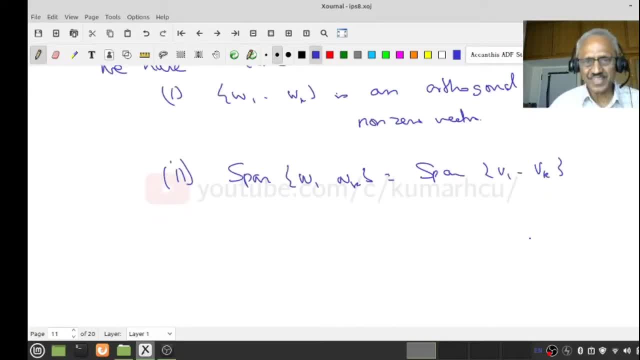 for induction. it's enough if i was done for induction. it's enough if i was done for, for for one, one, one, even two is good enough, but i just even two is good enough, but i just even two is good enough. but i just wanted to understand the geometry. 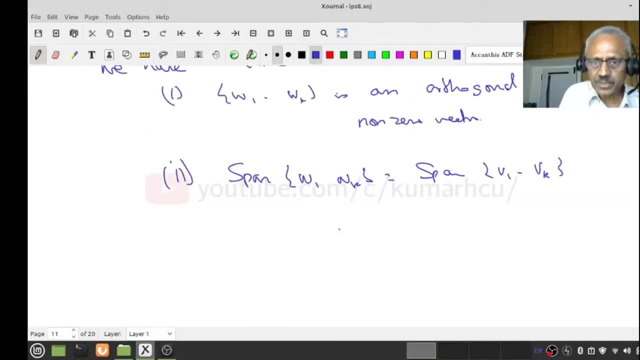 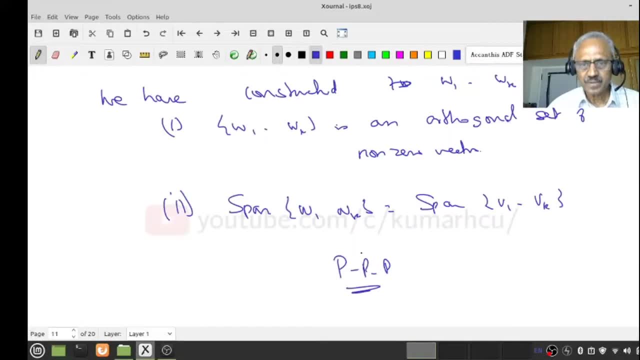 wanted to understand the geometry. wanted to understand the geometry. that's why very slow, is it clear? that's why very slow, is it clear? that's why very slow, is it clear? stage: i already have vectors w1 to wk. stage: i already have vectors w1 to wk. 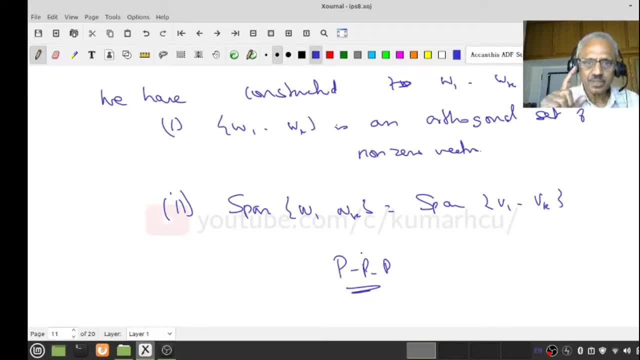 stage. i already have vectors w1 to wk. what are the properties this set w1 to? what are the properties this set w1 to? what are the properties this set w1 to wk is each one of them is non-zero and wk is each one of them is non-zero and. 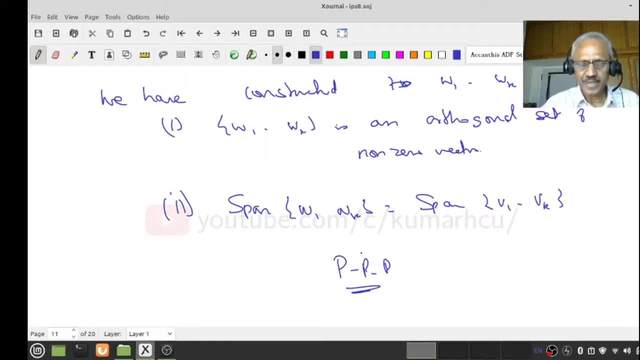 wk is: each one of them is non-zero and they are orthogonal to mutually. they are orthogonal to mutually. they are orthogonal to mutually, orthogonal to each other, orthogonal to each other, orthogonal to each other. and second thing is: and second thing is: and second thing is: they span a space. it's okay, that space. 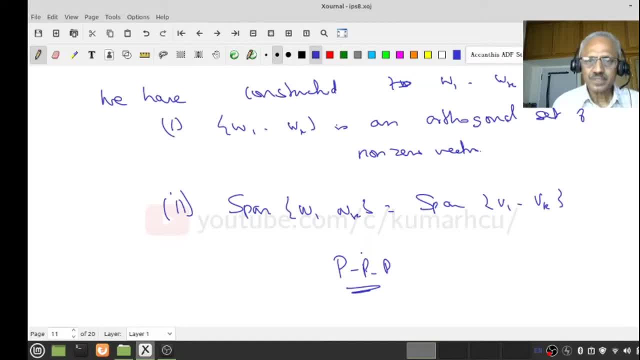 they span a space. it's okay that space they span a space. it's okay that space is nothing at the span of b1 to bk, is nothing at the span of b1 to bk is nothing at the span of bk. therefore, okay, cademption of the space. 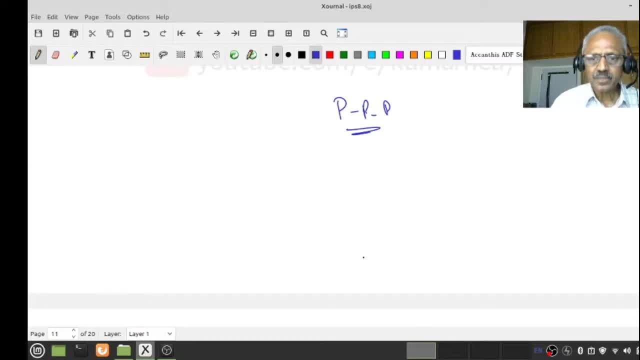 therefore okay. cademption of the space, therefore okay, cademption of the space board. is that all right board? is that all right board? is that all right? okay now. what is by induction? i have to do okay now. what is by induction? i have to do? okay now, what is by induction? i have to do, i have to consider. 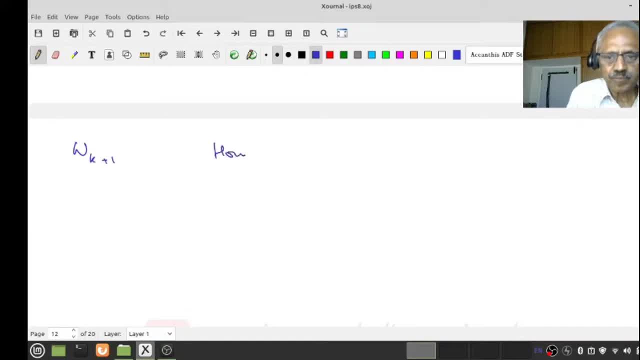 i have to consider. i have to consider wk plus one, how to construct wk plus one, how to construct wk plus one, how to construct, i'm sure, but if you have followed what i'm sure, but if you have followed what i'm sure, but if you have followed what i have said so far, 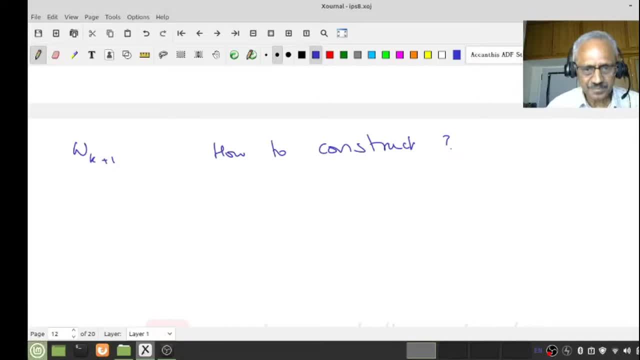 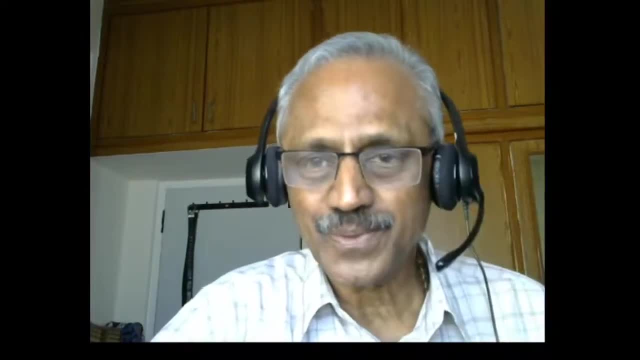 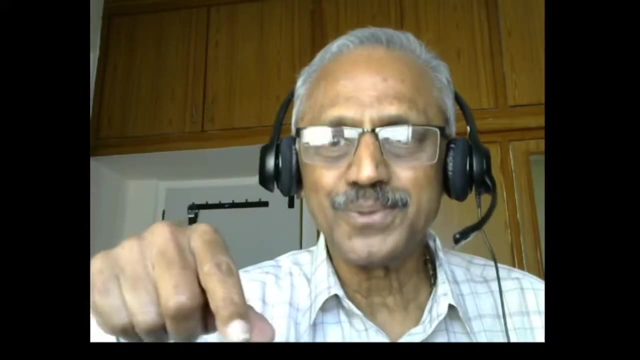 you should know. how do you think i you should know, how do you think i you should know, how do you think i should do wk, yeah, what do you have to do? yeah, what do you have to do? take vk plus 1, and what do you do? you are the only project: vk plus 1 onto w1, onto w2, onto wk. 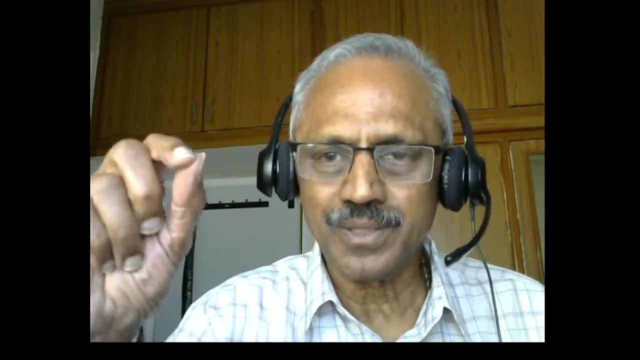 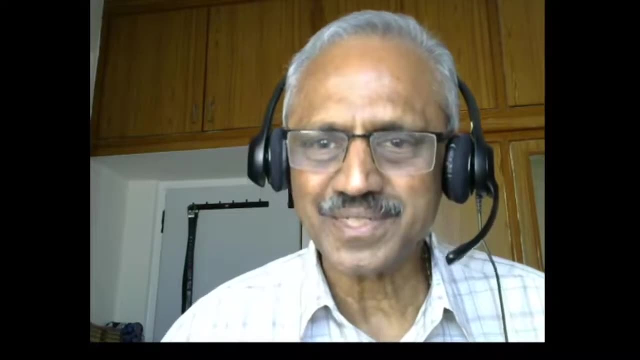 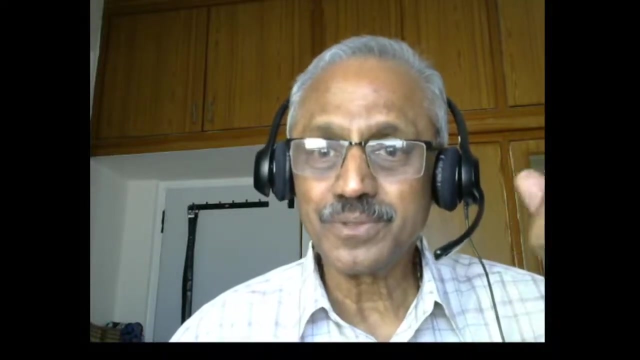 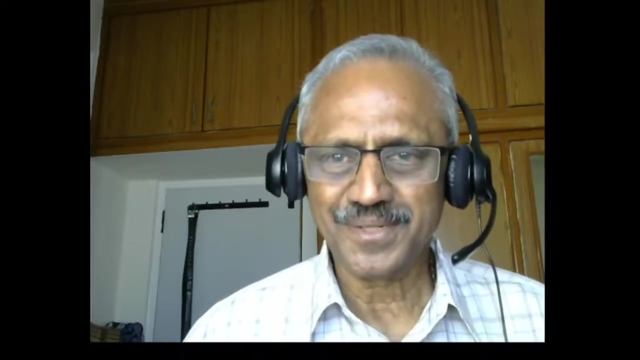 okay, compute that w1 component, w2 component, wk component and throw it out from vk. subtract it from vk, then i get a wk and i expect that wk will be 10 and further. it will be orthogonal to w1 to wk. is that clear, isn't it easy, okay, so don't watch the video now. pause it. try to do it. 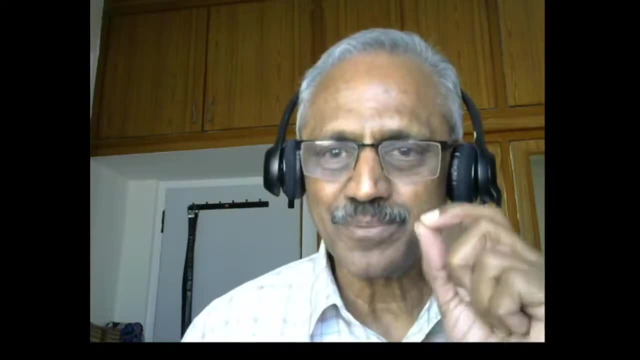 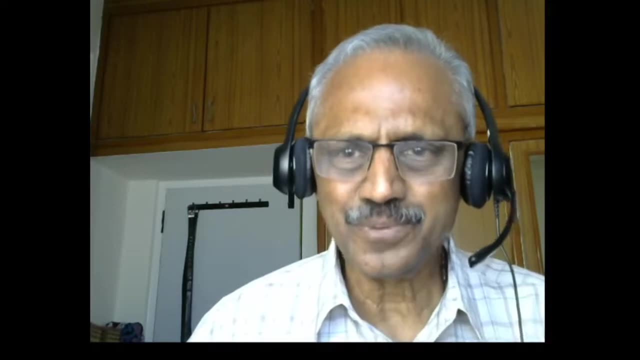 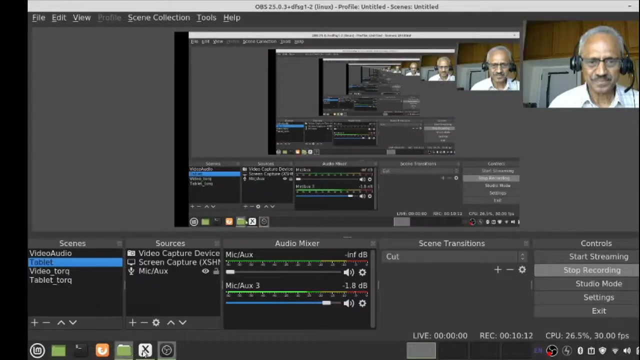 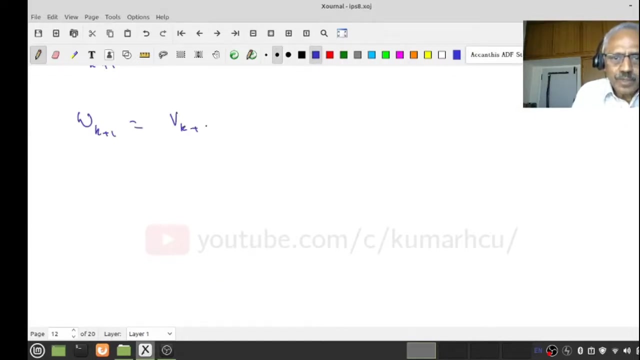 on your own write down, okay, the definition of wk plus 1. this will give you in immense confidence. yeah, try it in case, if you, if you struggle, the video you can again follow. right, do it. so how do you construct? so wk plus 1 is vk plus 1 and minus p1. of vk plus 1 minus minus pk of vk plus 1. 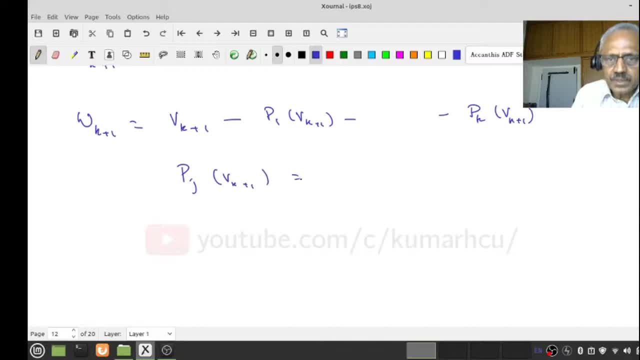 where pj of vk plus 1 is nothing other than p of wj of vk plus 1, that is dk plus 1, wj by wj, wj. and you see that if you do such things it becomes automatic. you do not remember. okay, is that clear. 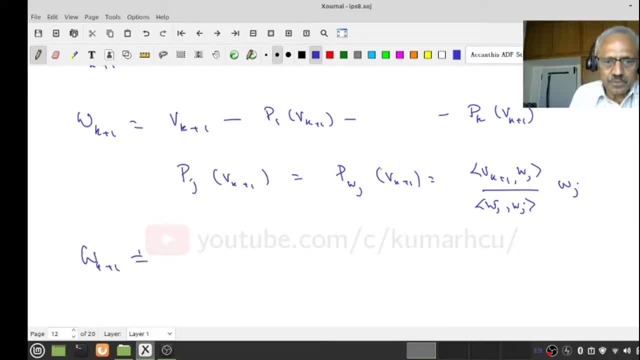 okay, now the first thing is: wk plus 1 is non-zero. why suppose zero? as usual, vk plus 1 will be a linear combination of this is w1- wk, right? but the w1 to wk lies in the span of v1 to vk, right? you understand that? therefore, vk plus 1 will lie in the linear span of. 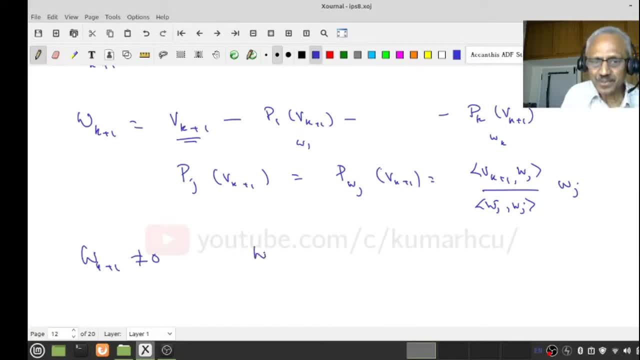 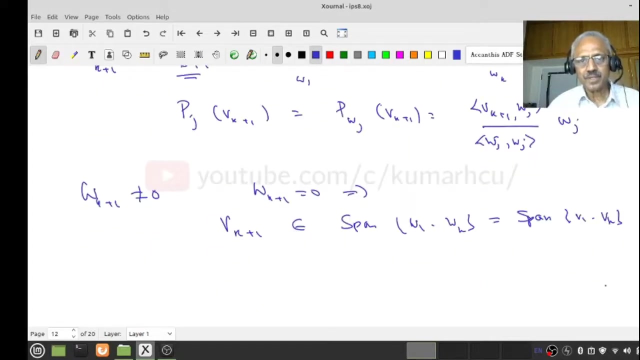 v1 to vk. do you understand this? if wk plus 1 is 0, that implies vk plus 1 lies in the span of w1 to wk. what is that? but this we know by induction hypothesis. this is the span of v1 to vk. that means what? vk plus 1 is a linear combination of vk to v1 to vk. that this is the contradiction. 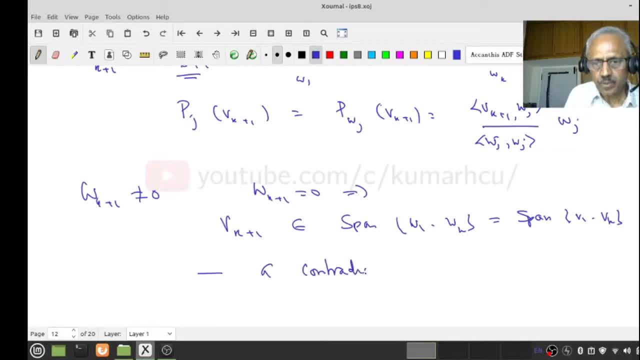 right why it's a contradiction? because v1 to vk is a subset of v1 to vn, which is linearly independent set. and remember, my k is strictly less than n. therefore we k even assume vk plus 1, it will be at most n. k plus 1 may be at most n, at most it may even be less. are you following? 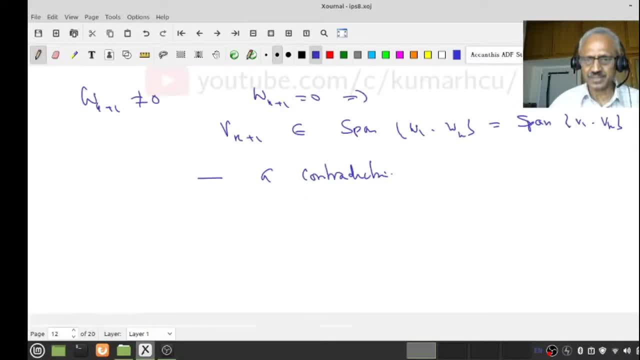 this is a non-zero. okay, therefore it's non-zero. and also, then, if the value of vn is greater than k plus 1 will be greater than n at most, n at most it may be less than k plus 1, and then vn is greater than n and therefore it is non-zero. 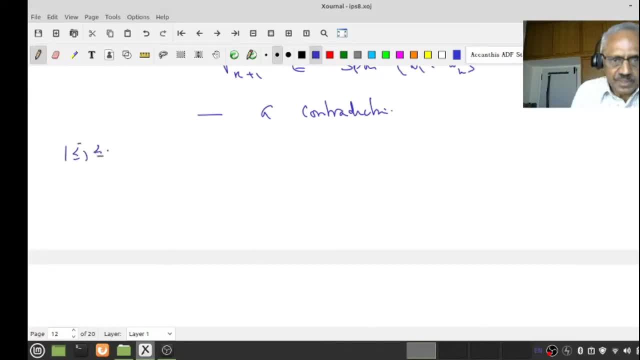 Then suppose 1 less than or equal to j less than or equal to k, right, What do I have to prove? I have to prove: wk plus 1 and wj is 0. But that's very easy. What is wk? 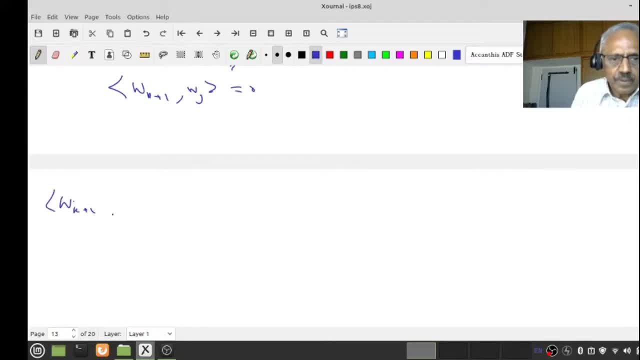 So this wk plus 1 inner product wj is vk plus 1 minus pj of vk plus 1 inner product wj. okay, So let us write it as pr: r equal to 1 to k, because this j is fixed now okay. 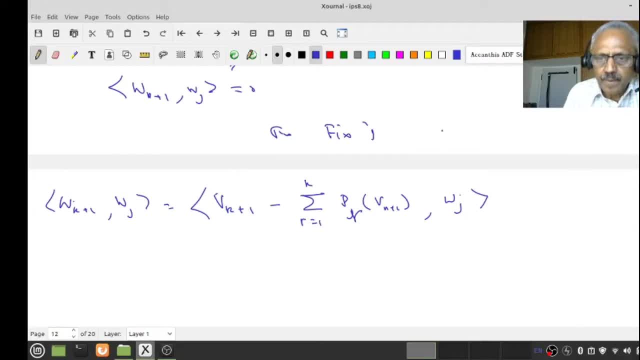 Fixed j. Okay, but what is this? This is vk plus 1 inner product with wj minus. okay. this again. do you remember my trick? Think of this as ordinary product. therefore, pk plus 1 wj and r equal to 1 to k. 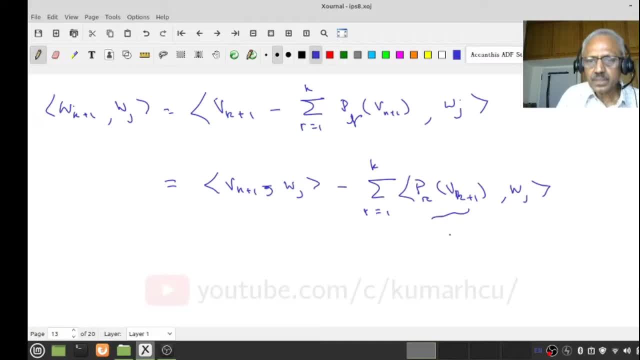 Now notice that this is okay. a multiple of wr Right, Therefore some multiple times inner product wr wj, okay. So then there is only one thing: service r is a running variable right. So unless r equal to j, then some scalar multiple wr wj will be 0. 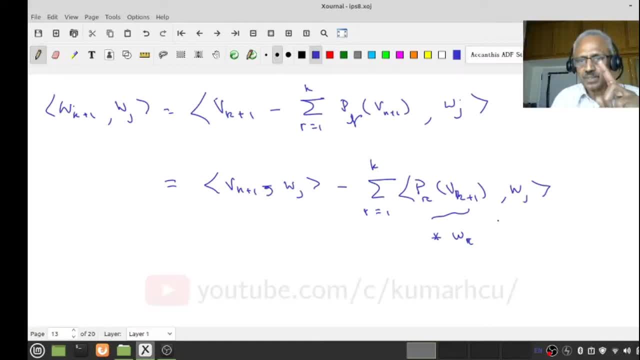 Therefore, what is left out? The only thing which is left out is r equal to j term. Therefore, this fellow is vk plus 1 inner product, wj minus pj. So vk plus 1 wj, yeah, But what is this object? 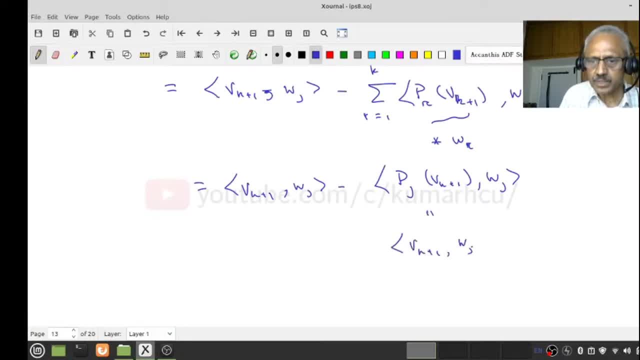 This object, we know is vk plus 1 wj, by wj, wj and into wj. this is this object: inner product with wj. So this is cancelled. therefore, this is 0.. Yeah, This is a scalar that comes out. this is a scalar that comes out. therefore, inner product: wj, wj. 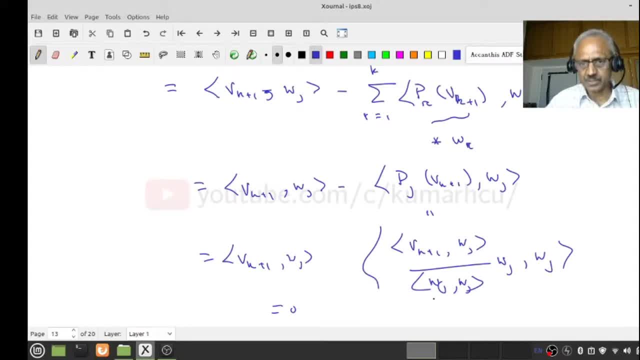 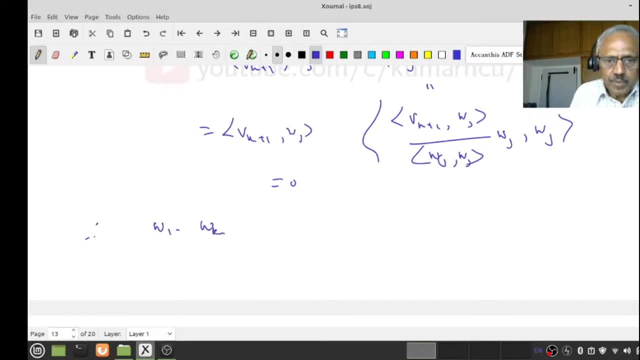 but there is a denominator: wj- wj. therefore, they get cancelled. therefore, is that all right? So what do you think I have proved? Therefore, w1 to wk plus 1 is an orthogonal set, Non-zero vectors. 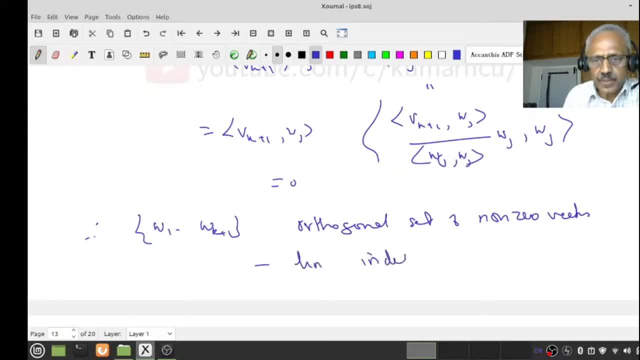 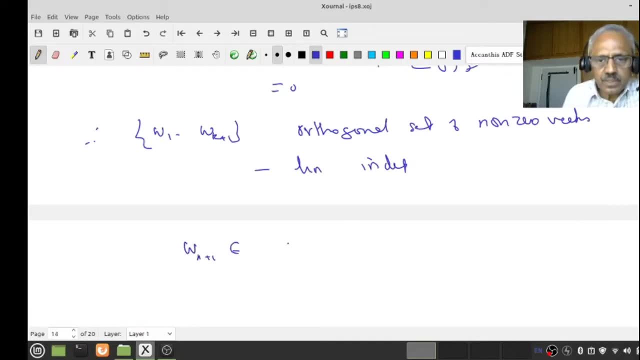 Right. Therefore this is linearly independent. All right. Now again, notice that wk plus 1 is lies in the span of v1 to vk plus 1.. And w1 to wk lies in the span of vk to vk. therefore, it lies in the span of v1 to vk, vk plus 1.. 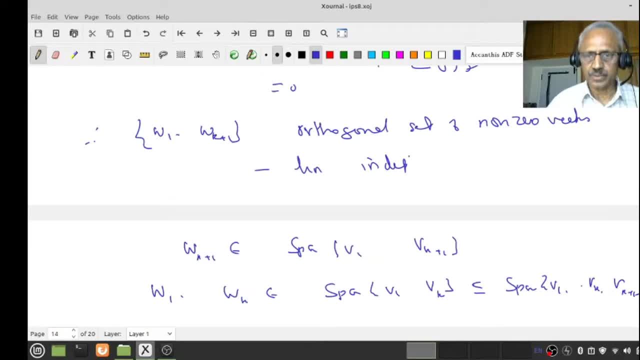 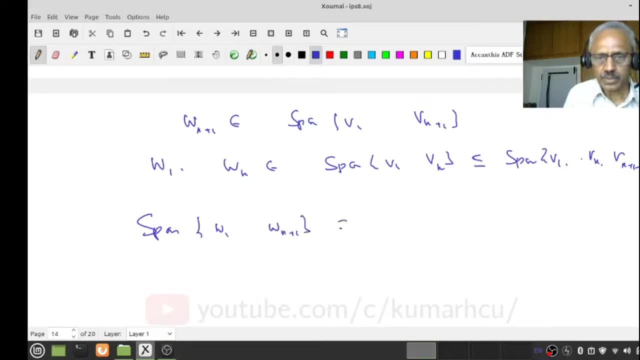 All right. Therefore, what do you think I have proved? I have proved Span of w1 to wk plus 1 equal to span of u1 to vk plus 1.. How did I prove that? Because this is linearly independent and therefore dimension will be k plus 1, whereas this dimension is k plus 1.. 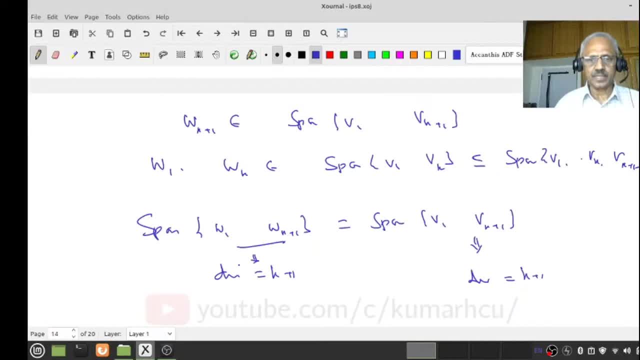 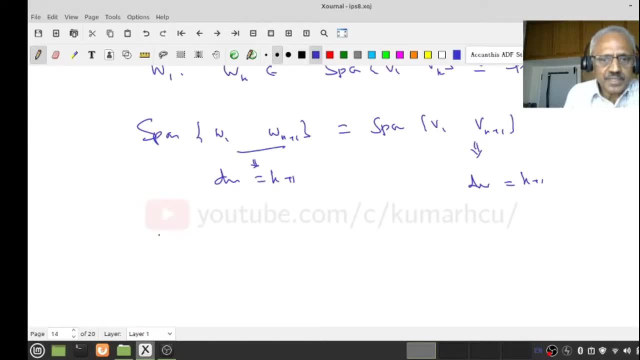 Right, And therefore this is a subset of that and therefore they are equal. it is the same logic as you had done. Okay, So now by induction out of 1 to n, I have to. therefore, okay, by induction, we have produced vectors w1 to wn in V, such that 1, w1 to wn is an orthogonal set of non-zero vectors. 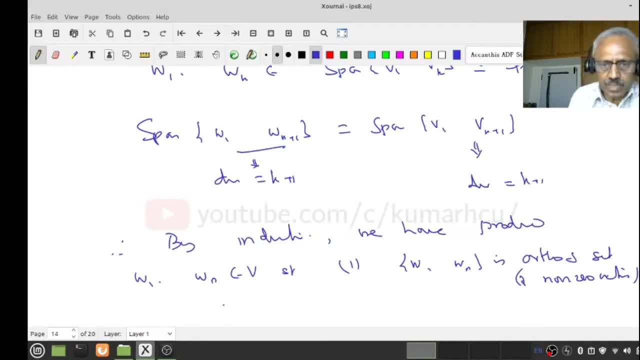 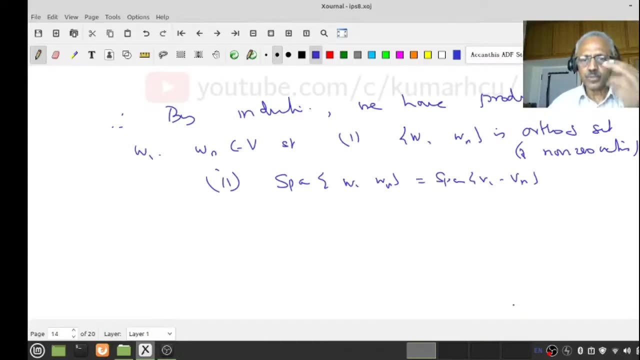 But non-zero vectors will actually come from the second one and the span of w1 to wn equal to span of v1 to vn. But let us you know, v1 to vn is a basis and w1 to wn is also has exactly n ml and its span is the same as this. 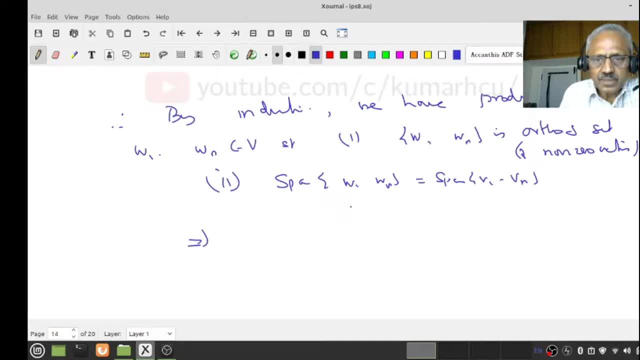 Therefore, what do I conclude? You understand that This is n vector, these are n vector, this is the dimension, Okay, And these n vectors Span this. So what is the conclusion? w1 to wn is a basis. 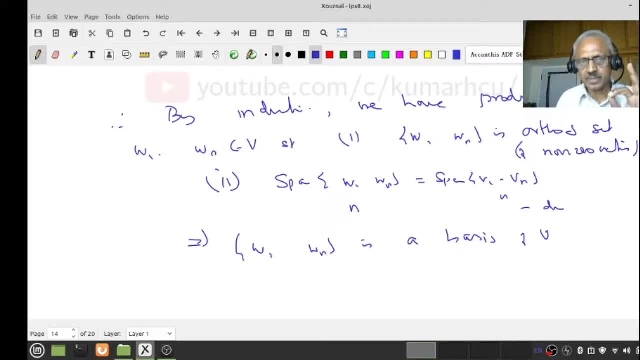 Are you sure about this? Make sure you are understanding. Yeah, If I have an intentional space, if I have some vectors, let us say something. okay: u1 to un which span the space, then u1 to un should be linearly independent, as well as you know, non-zero. 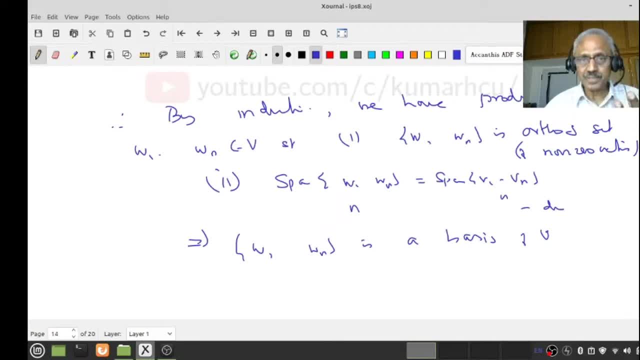 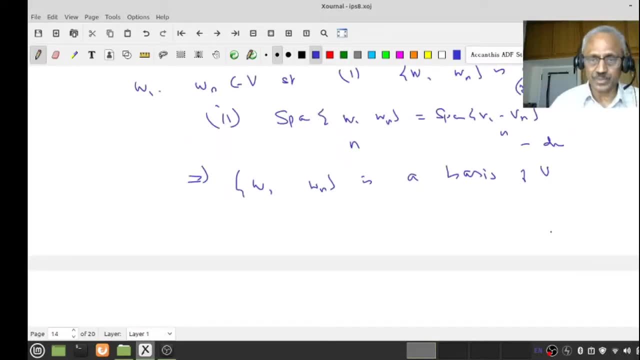 Okay, So if I have an intentional space, then u1 to un should be linearly independent as well, as you know, non-zero. It must be a basis, Okay, But we had already shown it's a linearly independent, but what we are showing is actually a basis. 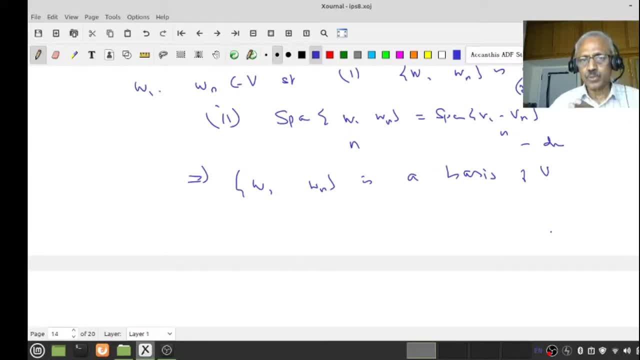 Right, Because, remember w1 to w1, they are all mutually orthogonal, They are non-zero. Since they are non-zero, we know that set is linearly independent. Therefore, this is the set: w1 to wn is a set which is linearly independent, having n elements. 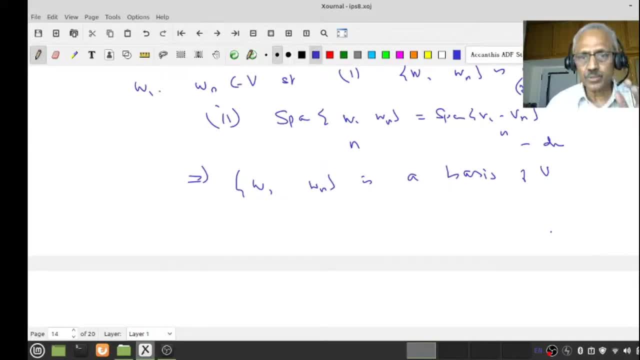 But the dimension of the space b is n. Therefore, w1 to wn, W1 must be basis, So there are a lot of ways of seeing. Okay, Try to think Okay. So what do I know about this? 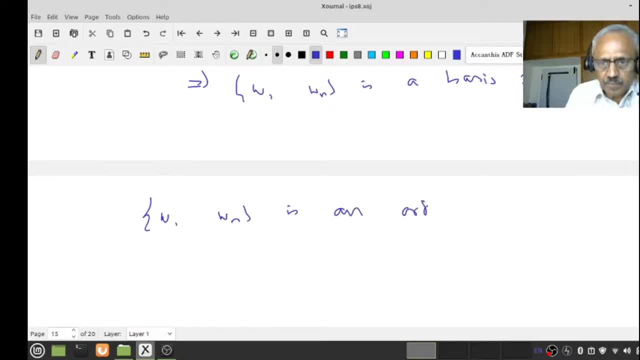 W1 to w1 is an orthogonal basis. Now how do I get orthonormal? Remember these are all basic elements. Therefore, w1, w2, w1 are non-zero. Therefore, define uj to be wj by norm of wj. 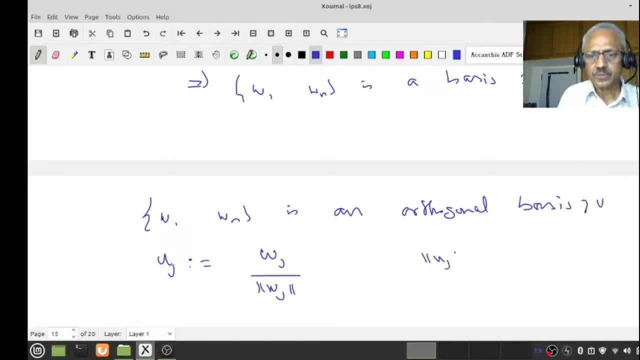 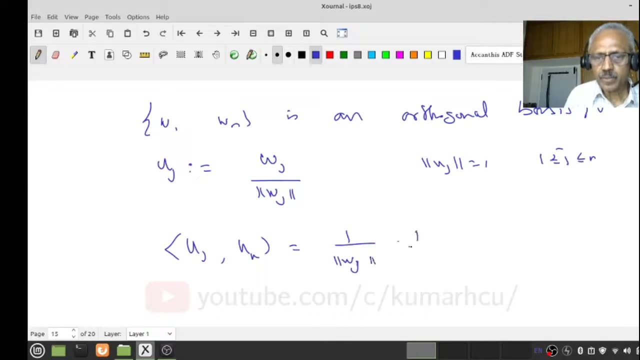 Right, Then uj is always 1 for 1, less than or equal to j, less than or equal to n, And what do I know? And uj and ukr, this is norm of wj and 1 by norm of wr, and wj, wr. 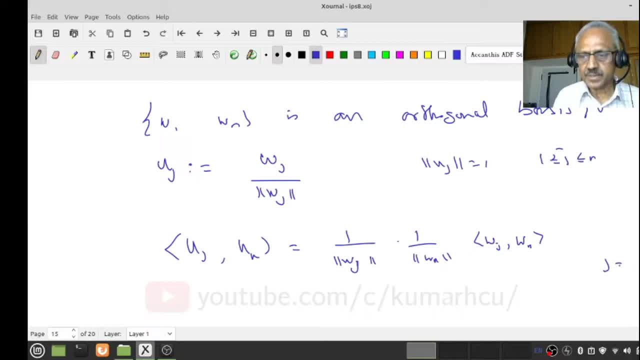 Is that okay? And if j is not equal to r, then this is zero. Okay, j equal to r. this is wj, wj And this is also wj. this is also wj. Therefore, 1 by norm, wj squared that cancel. 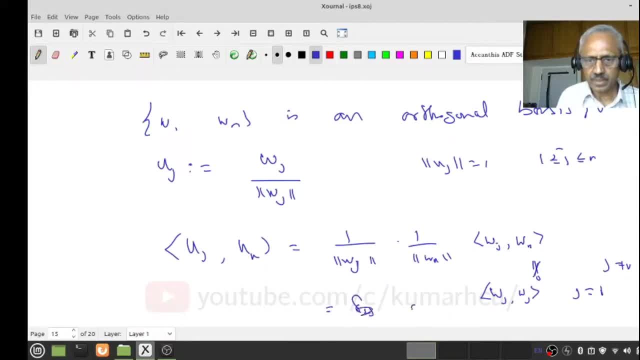 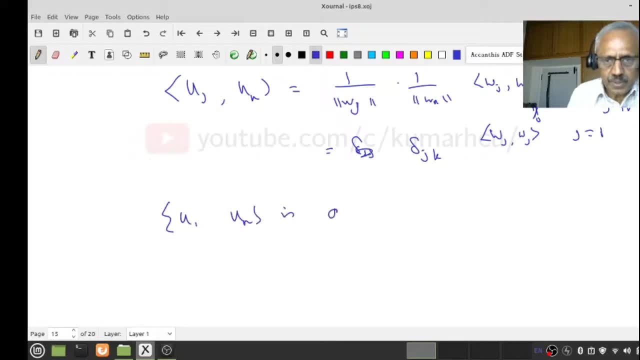 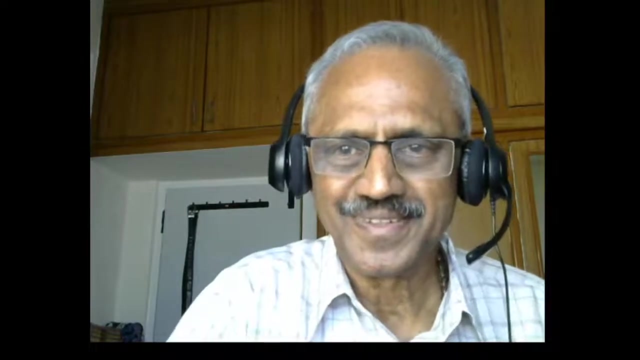 Therefore, I get 1.. So this is delta jk. You understand that. Therefore, u1 to wn is an orthonormal basis. That's it. We proved it. How did you like the proof Isn't it easy. 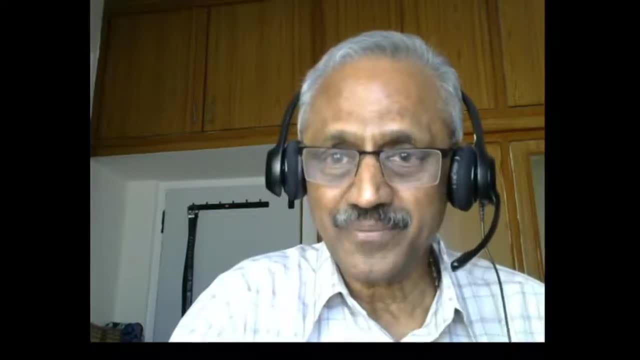 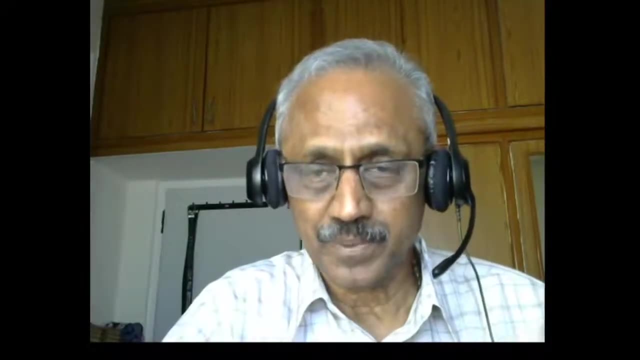 Because the geometry helped us how to write the expressions, and we also know how to do that. The most crucial thing is look at the way the induction hypothesis is formed. Okay, When you want to learn, please go through it twice. Okay, Our assumption is at the kth stage. 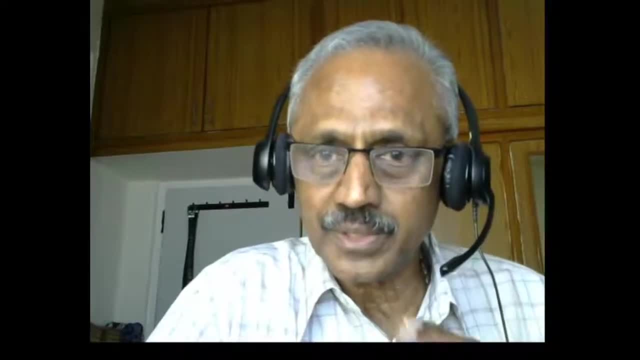 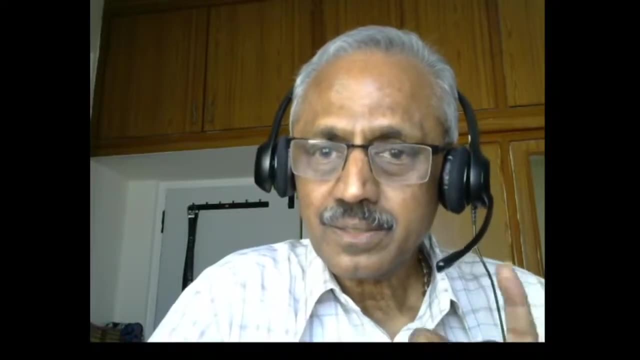 What is our assumption? I have considered w1 to wk And this set has two properties. What is the two properties? None of the wj is zero And that set is the wj and wk are orthogonal to each other. 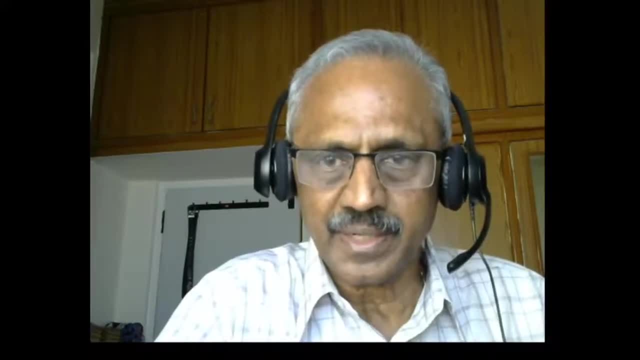 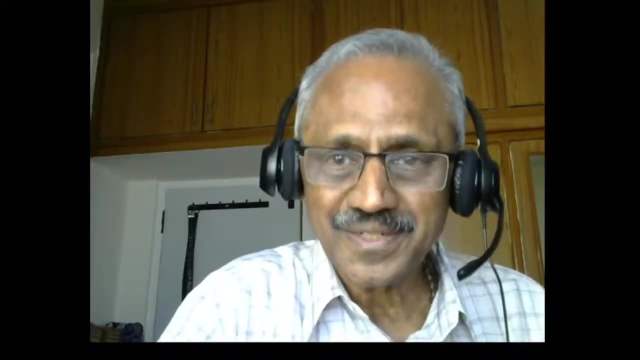 If j is not equal to you know wi and wj, for i not equal to j. they are perpendicular to each other. Right, It's an orthogonal set of non-zero vectors. Second thing is most very crucial. That is why I built up v1, v2, v3 and w1 to ww. 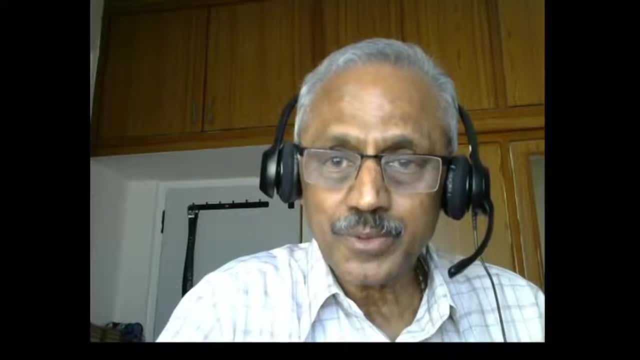 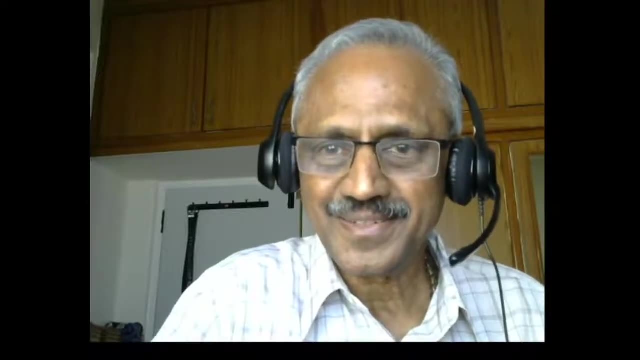 I went slowly. What did we show? The linear span of w1 to wk is exactly the linear span of v1 to vk. All right, You understand the proof. Please go through it. At least go through twice. You will be surprised. 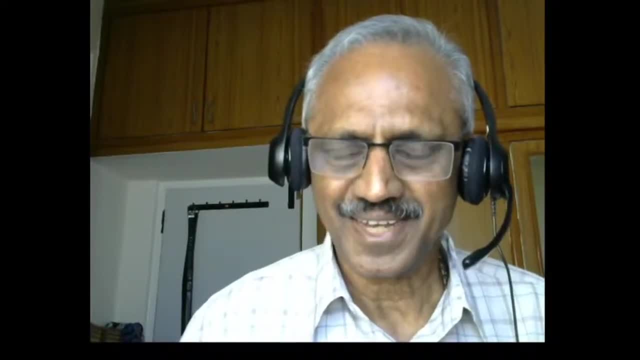 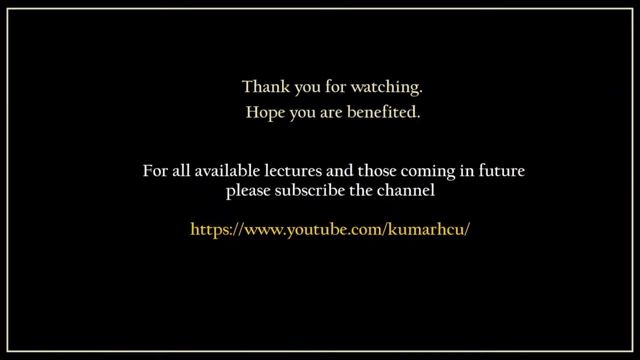 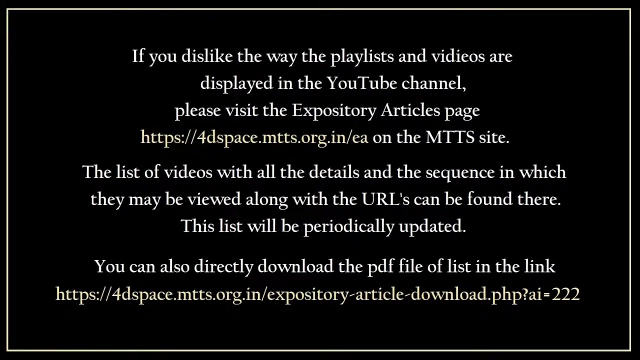 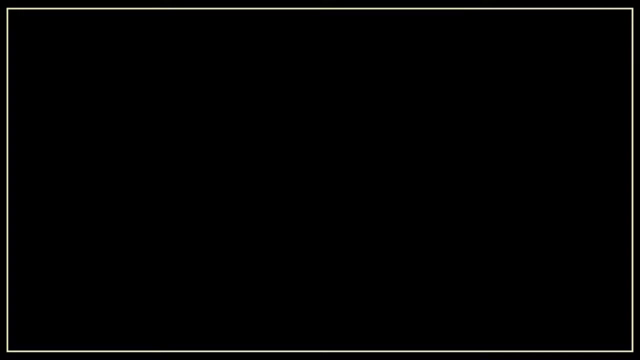 At any time, you can give the proof. Okay, I hope you enjoyed it. We will meet again, Thank you.